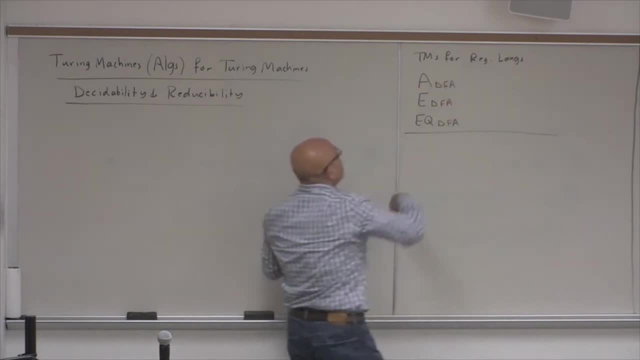 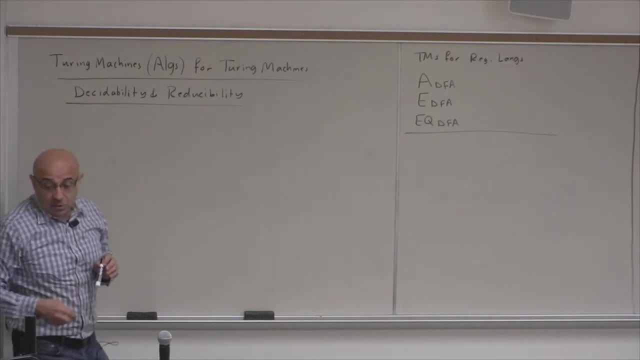 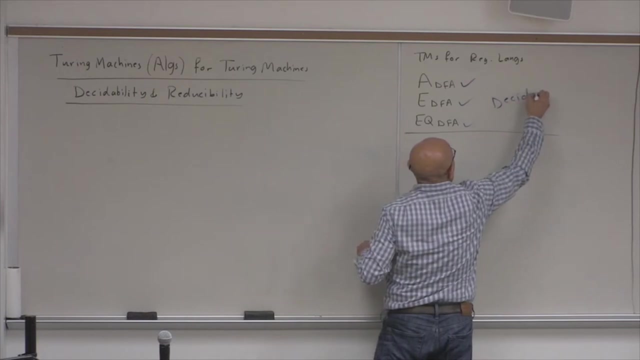 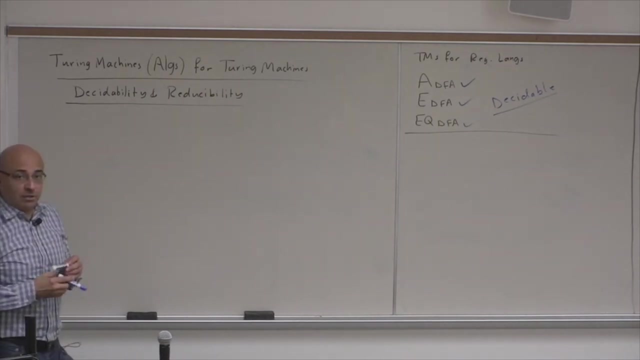 And for these problems about regular languages, could we find Turing machines or not? Yes, Yes, So we found Turing machines. So all three were decidable. So for each one of these, we described the Turing machine, or an algorithm that is guaranteed to terminate. 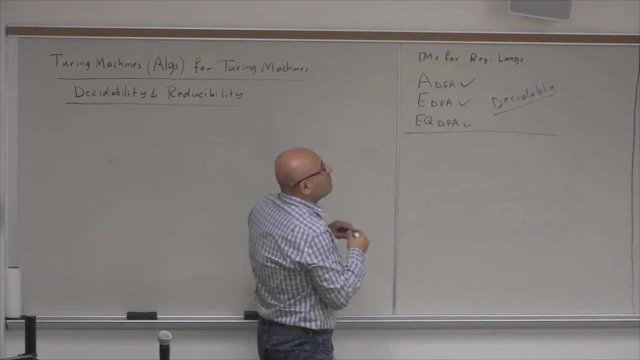 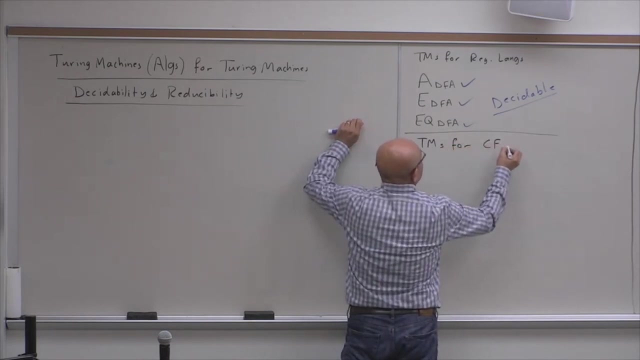 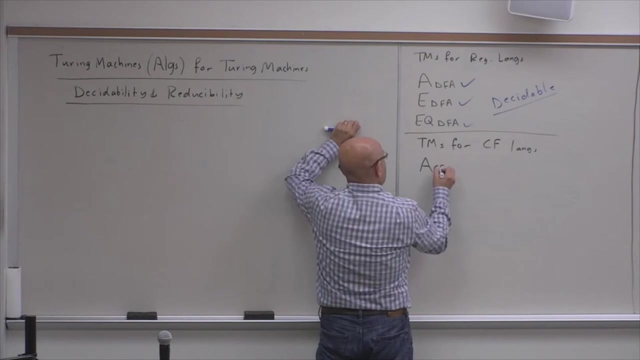 in regular time, in finite time And Turing machines for context-free languages. that was the focus of last lecture: context-free languages. So we talked about A CFG E, CFG and equivalence of CFGs. So this is. 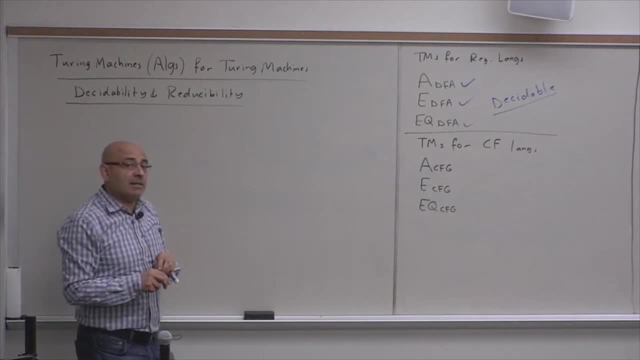 the acceptance. Okay, So what we found about E E CFG and E E CFG is that it DXA, which is the equivalent of DFA. is that it's the same as Clik. It's the same as Clik. So this is. 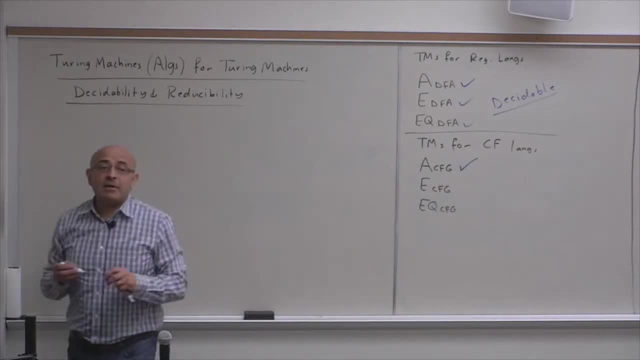 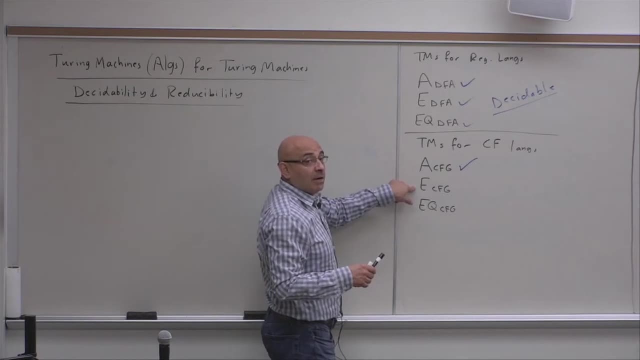 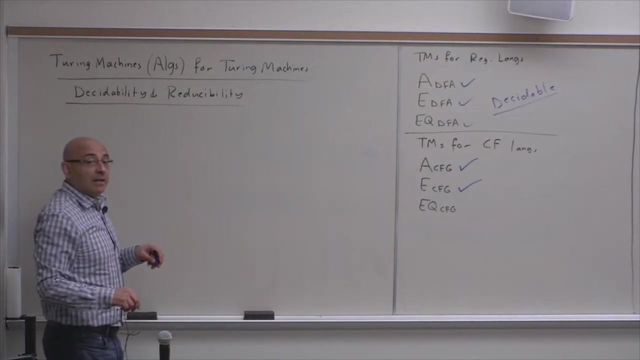 the same as Clik, And so we found E, I E C, that it's the equivalent of C C 12.. Okay, So we found that E E C DFA, which is the equivalent of C DFA, is not present. 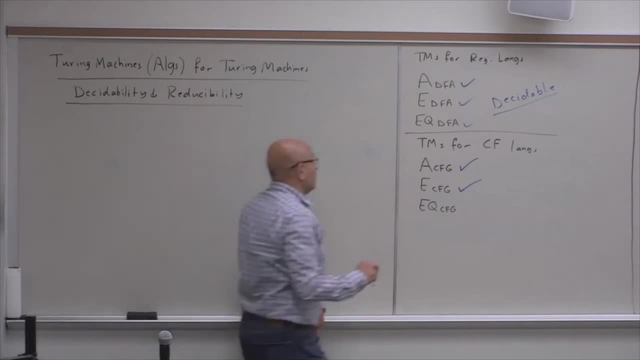 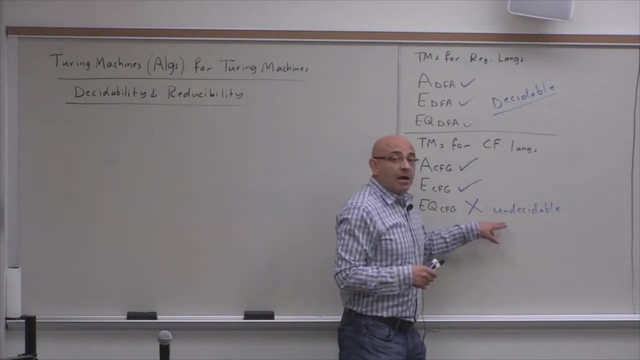 Was this decidable or not? No, it was not decidable, so undecidable. In fact, you know that was the first undecidable language that we studied. So undecidable language means a problem that cannot be solved using algorithms. 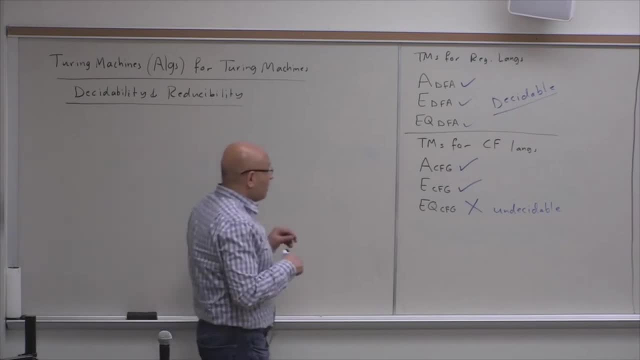 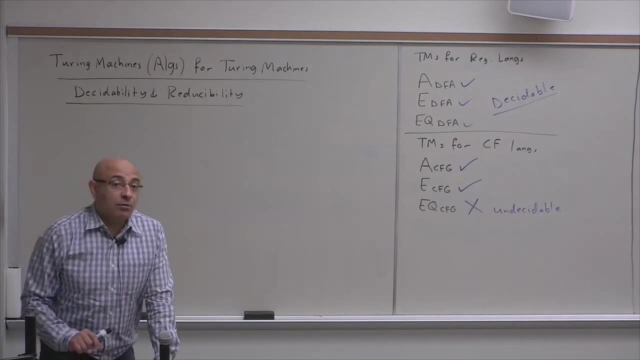 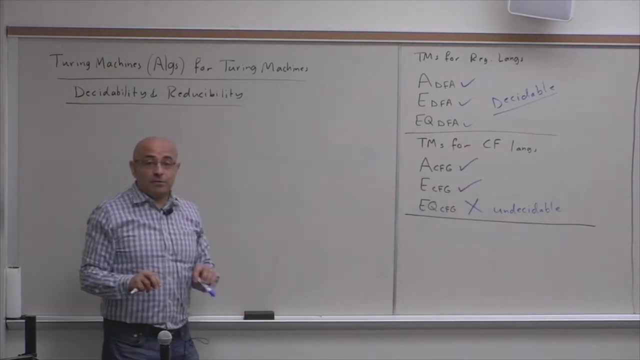 So there is no algorithm. You cannot come up with an algorithm that will take two context-free grammars and determine if they are equivalent or not. okay, Of course we did not prove this, but we just attempted to construct to use the same technique that we used. 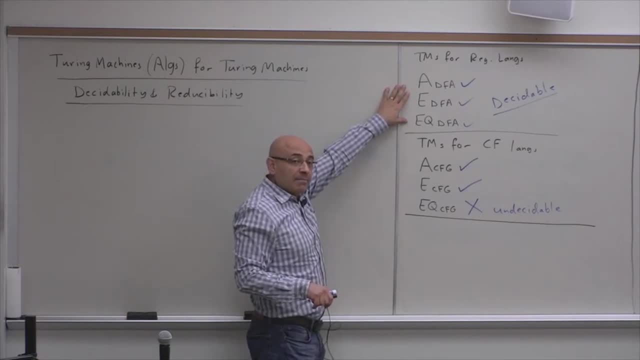 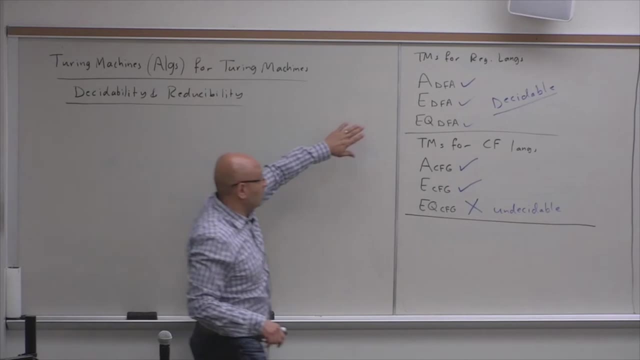 for regular languages. We tried to use the same technique, but we failed. because? why did we fail To use the same technique that worked for regular languages? Yeah, because context-free languages are not closed under intersection and complementation. So today we're going to look into Turing machines. 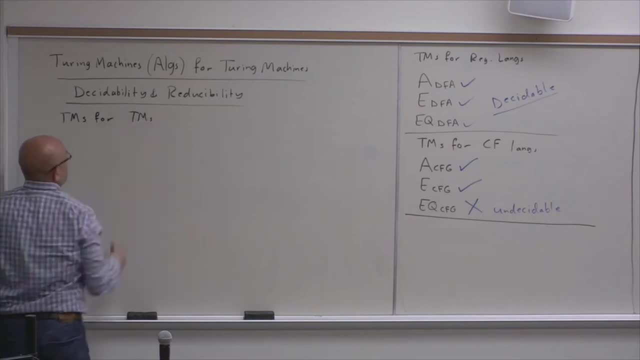 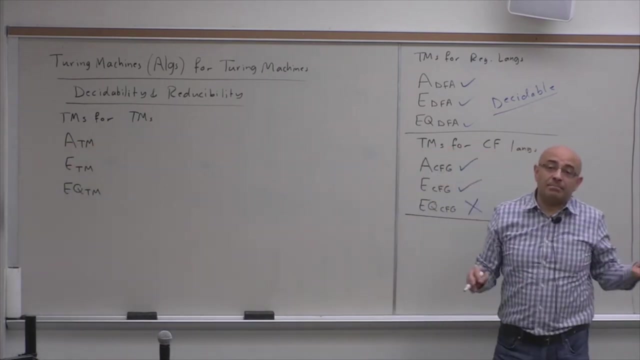 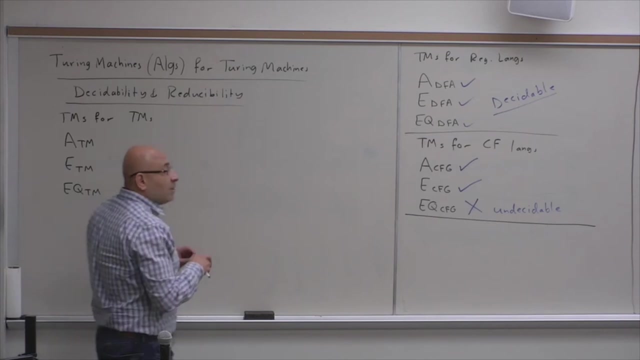 for Turing machines. So accept Turing machine, empty Turing machine and equivalence of Turing machines. So now a Turing machine. you can think of a Turing machine as a program. In fact, you know, in this lecture I'm going to focus. 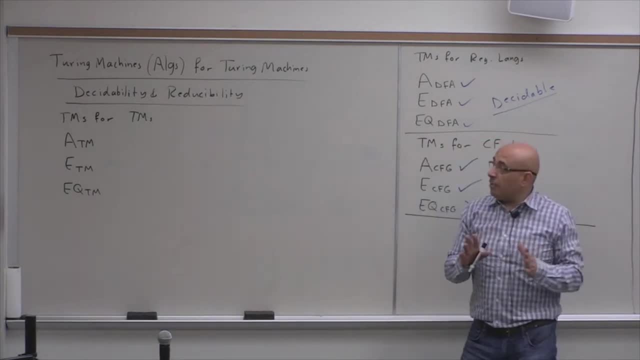 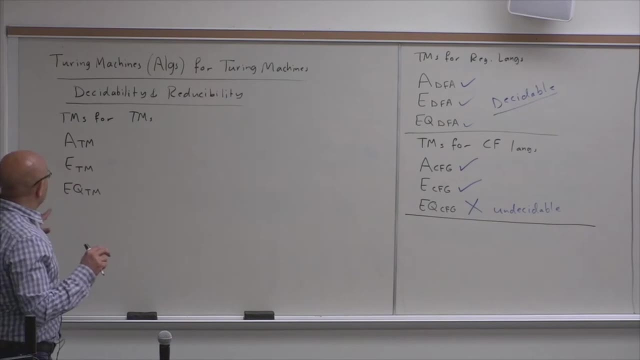 on the intuition. So I'm going to focus on, you know, the. I will most of the time view a Turing machine as a program, not as a, you know, an abstract Turing machine. So that it's you know this presentation makes. 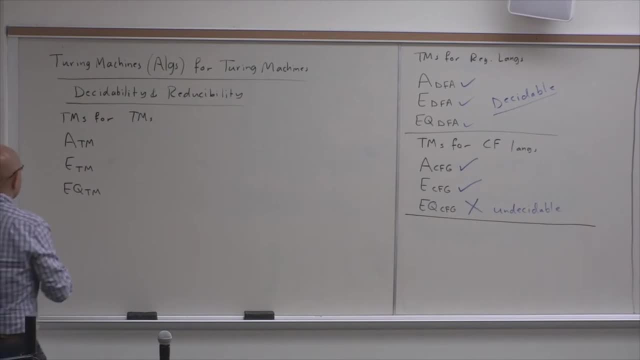 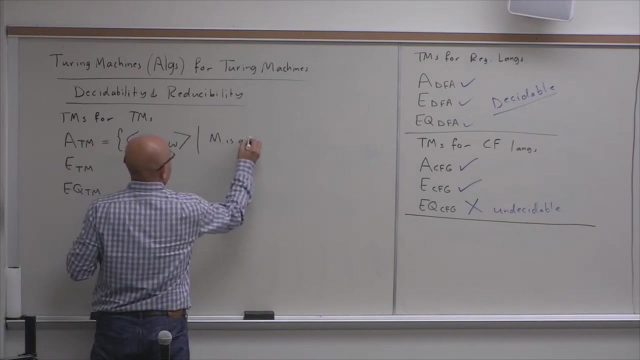 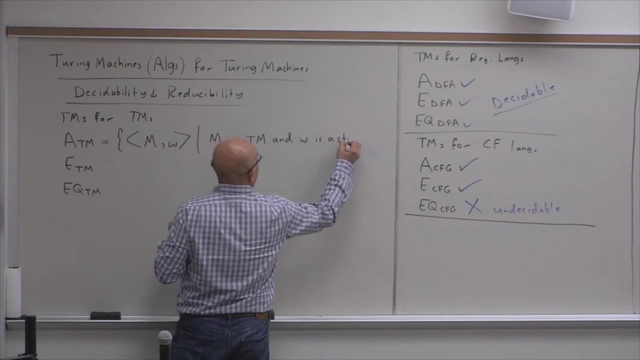 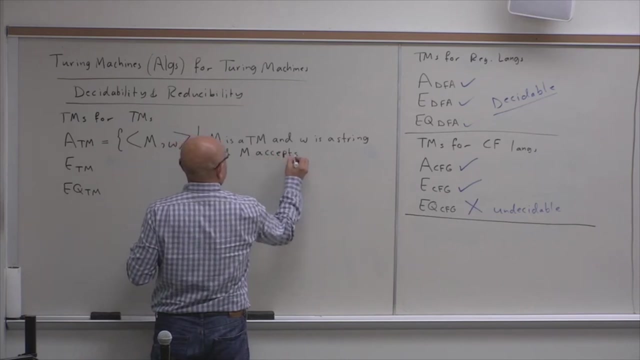 is more intuitive. So ATM is you are given. it's the language where you are given a Turing machine, M, and a string, W. So M is a Turing machine And W is a string and M accepts W. Okay, and ATM is checking. 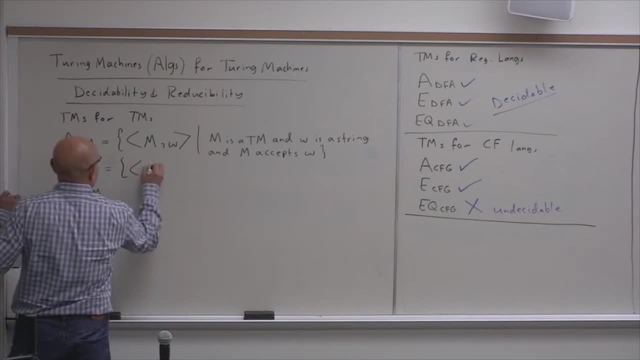 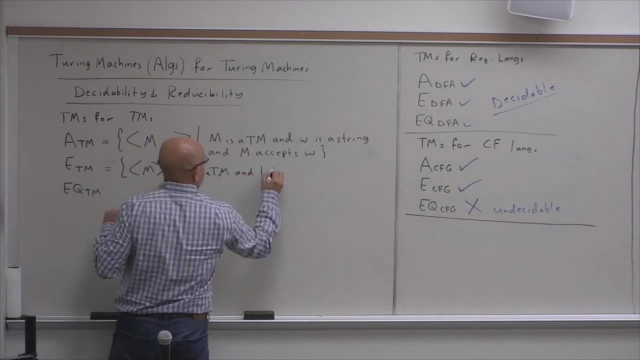 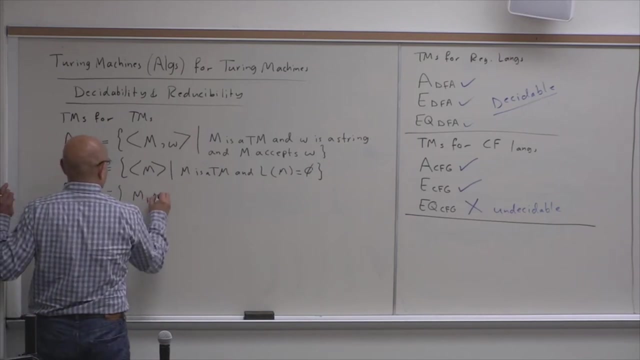 if a Turing machine is empty, so this is going to be M. M is a Turing machine And L of M equals phi And this is the equivalence of Turing machines. So it's M1 and M2.. You are given two Turing machines: M1 and 2, M2.. 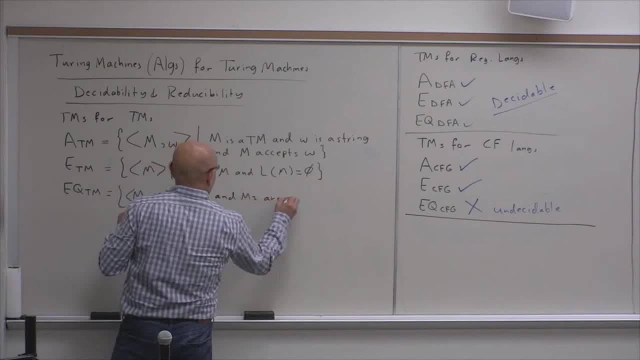 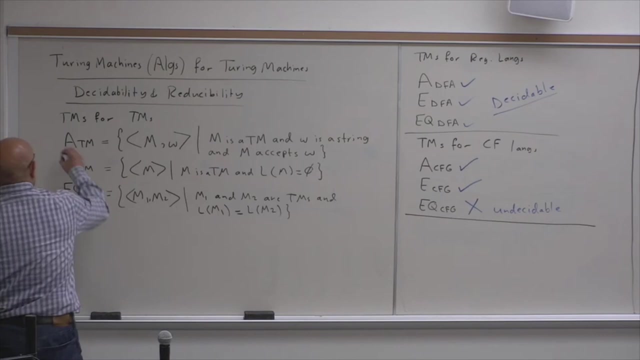 M1 and M2 are Turing machines And the language of M1 equals the language of M2.. I'm sorry we're going to focus on this today. So the so today we will focus on showing that ATM which is determining. you know, given a Turing machine, 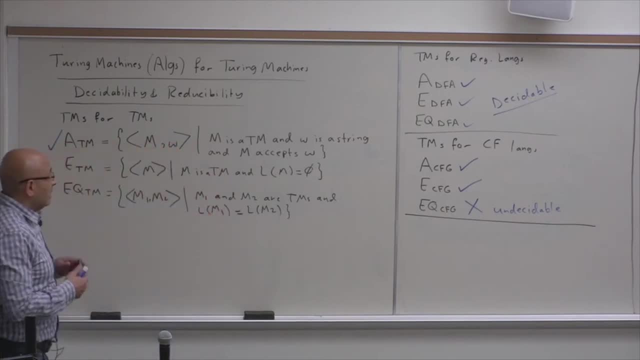 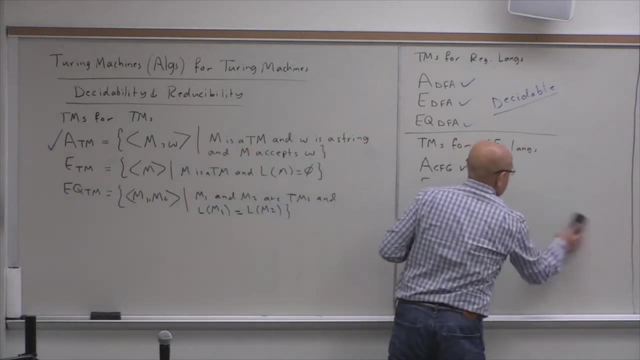 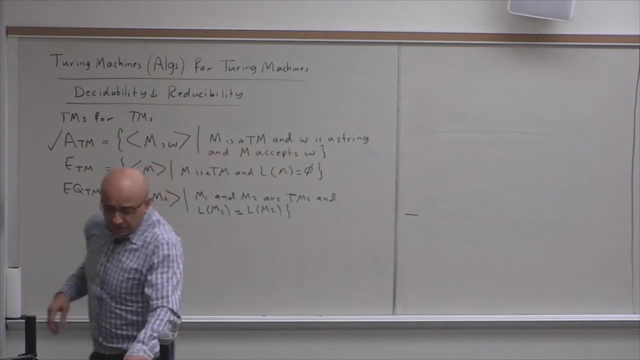 determine if it accepts a given string or not. Now let's think about this in terms of programs, not Turing machines, so that it makes more sense and it's more concrete. So before I start, you know, can anyone describe this problem? 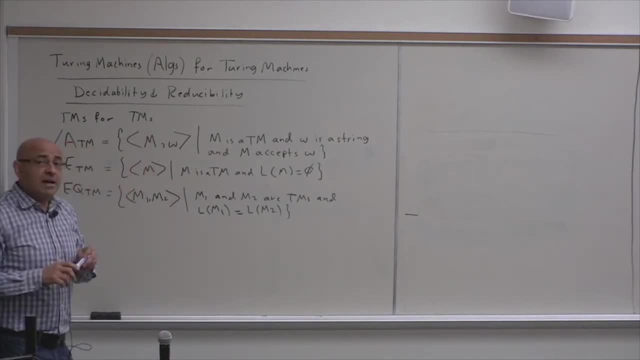 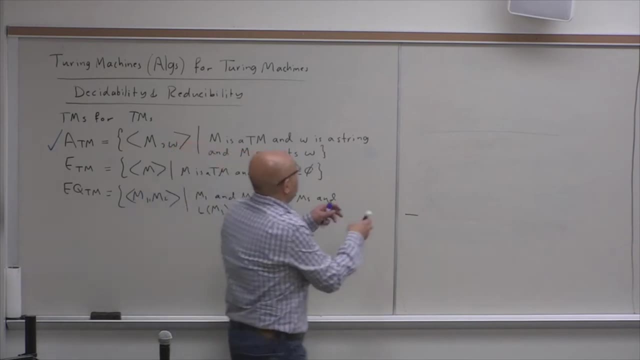 in terms of programs. So a Turing machine. think of a Turing machine as an algorithm. and an algorithm is implemented using a program, using some programming language. so program. Think of the Turing machine as a program written in some programming language. 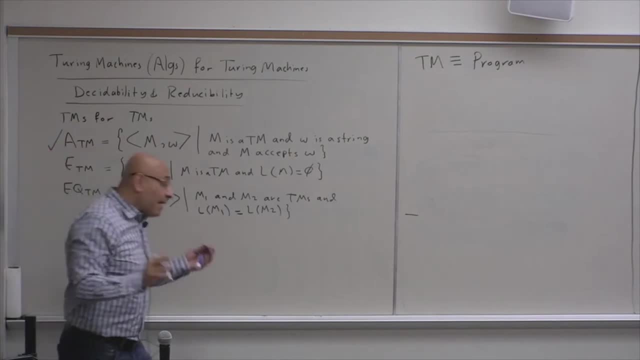 in a general purpose programming language or in fact a Turing complete programming language. So you know, We say a Turing complete programming language is a programming language that can do all the, that has all the features that a Turing machine has, You know, of course, a modern operating. 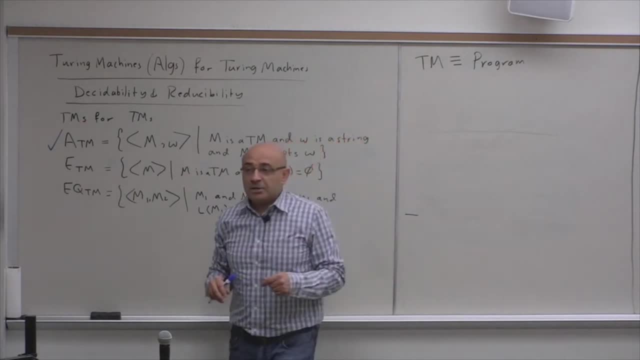 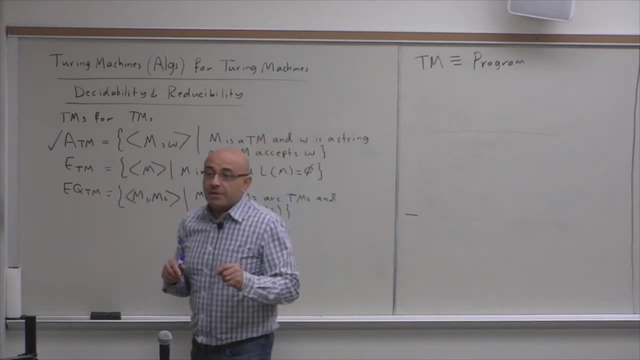 a modern programming language is much, much easier to program compared to a Turing machine. You know the Turing machine is a primitive, theoretical model. It's not something that that can have any practical value today. You know the Turing machine is a. 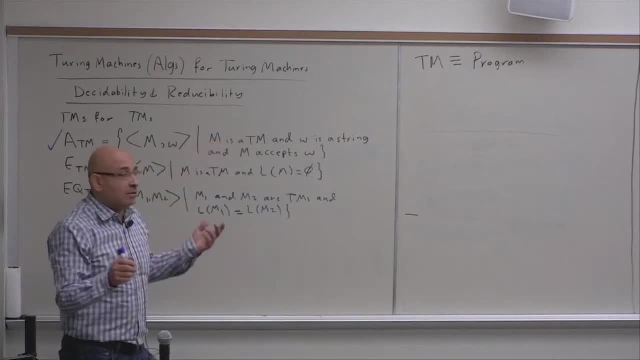 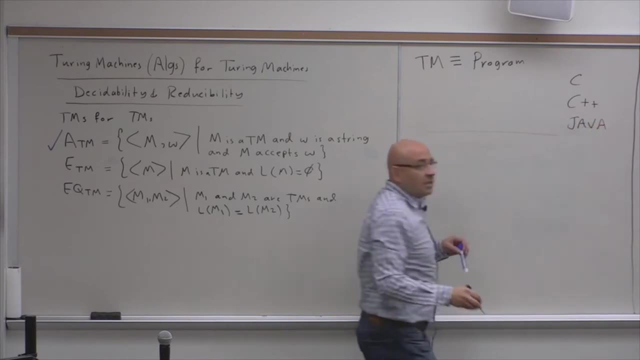 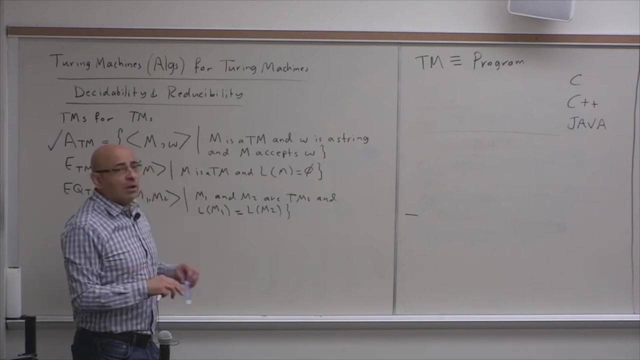 but a program written in one of the languages that we are familiar with, like, you know, C, C++ or Java, general purpose programming language. You can think of it as a, as a Turing machine. You know it's. it has all the features. 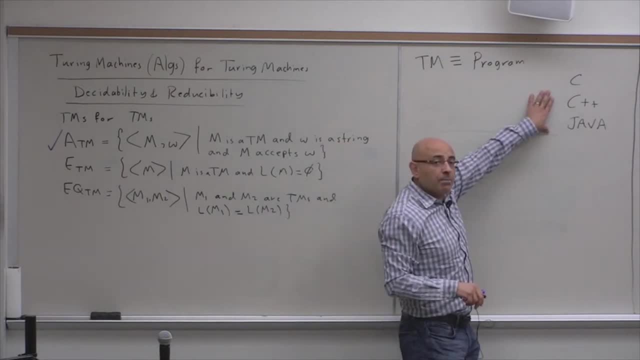 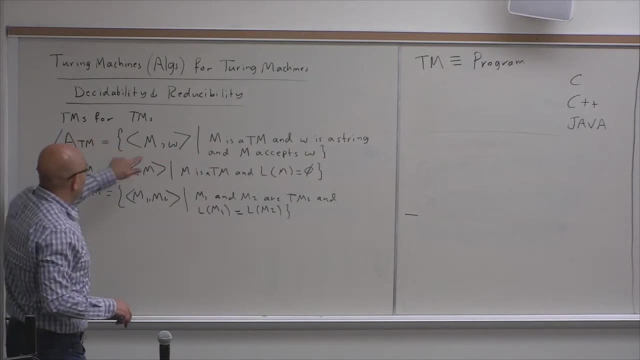 It can. you can do with it anything that a general purpose computer can do. So, thinking of a Turing machine as a program, what does this problem mean? What is it like in terms of don't use Turing machines, use programs, use the word program. 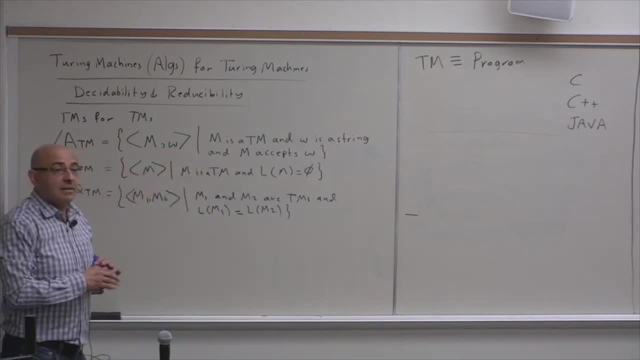 What does this problem, ATM mean? It means you are given. so this is a. we are looking for a program that takes another program- okay, and an input to that program and determines if the output is going to be accept Or reject. 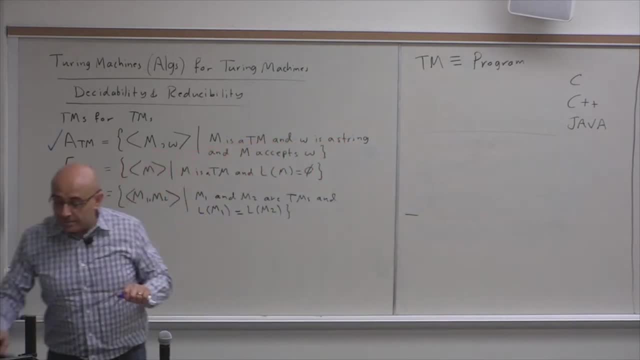 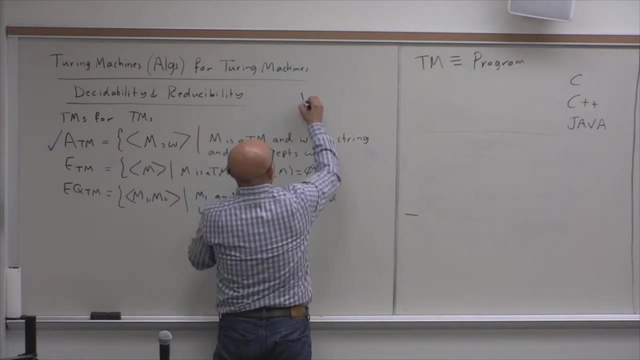 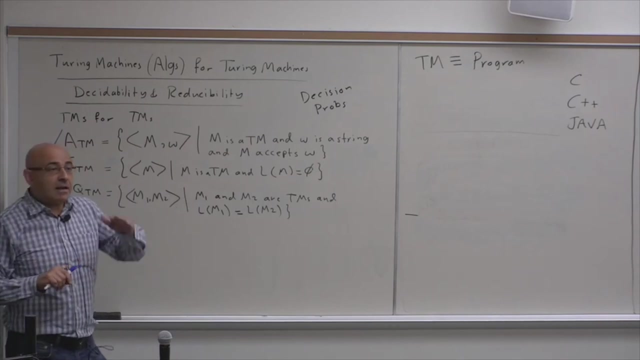 So the programs that we are talking about here are programs whose output is yes or no. So we're talking about programs that solve decision problems. So at this point we are talking about a program that takes an arbitrary input and the output of that program is yes or no. 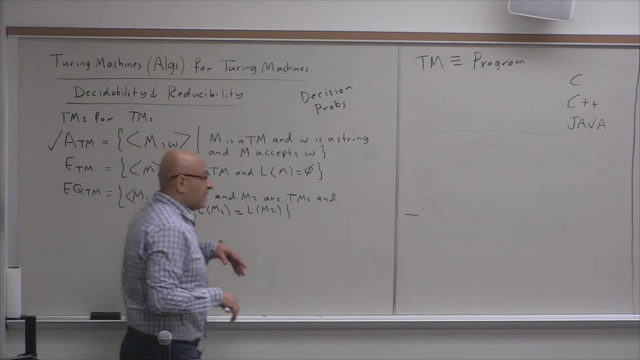 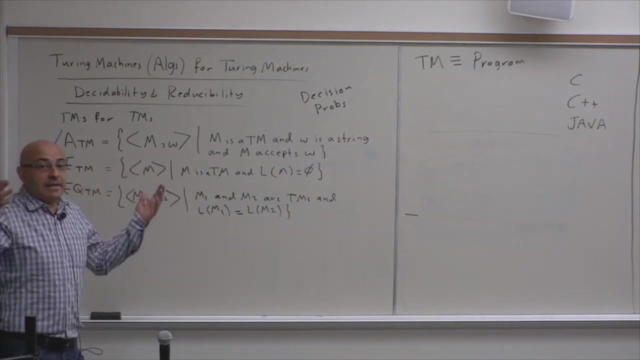 So like a program that takes a graph and determines if the graph is connected, Or a program that takes a graph and determines if the graph has a cycle or not. Okay, You know. or you know a program that you know that takes two finite automata and determines: 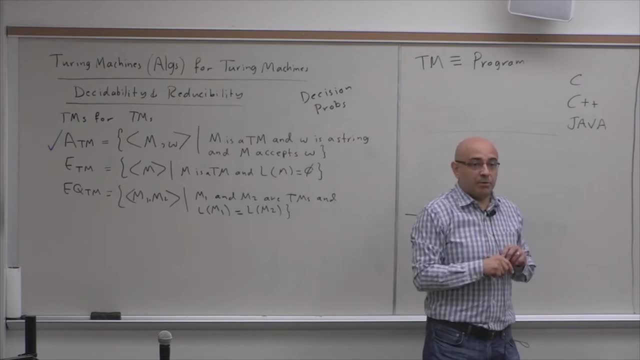 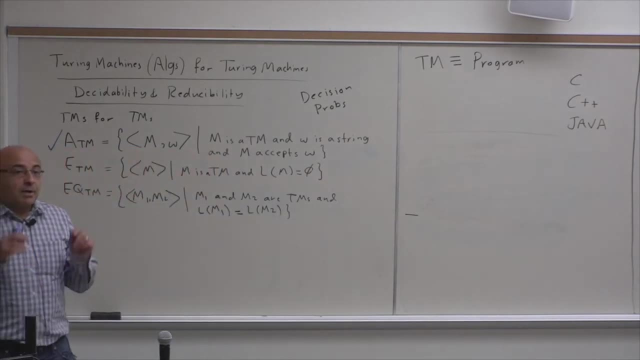 if they are equivalent or not. We know that we can write such a program. We can write a program that takes two finite automata and determines whether they are equivalent or not. But we know that we cannot write such a program. So we cannot write a program that takes two context-free. 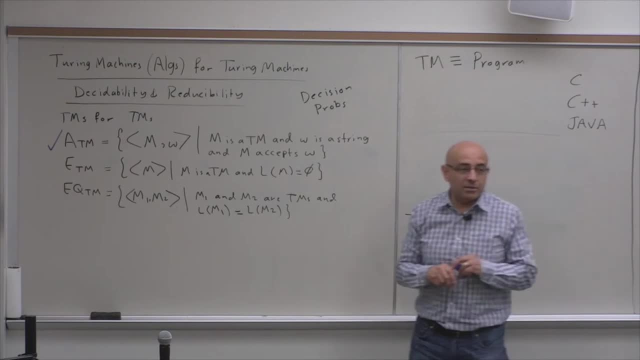 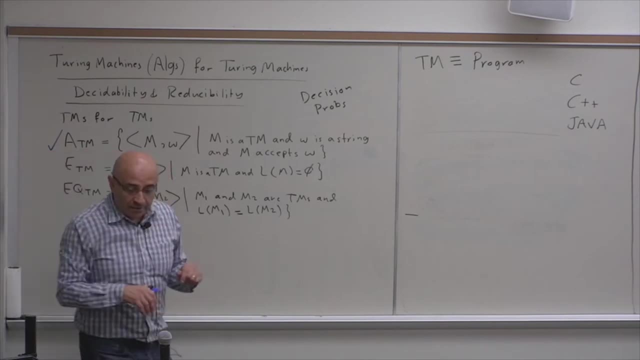 grammars and determines if they are equivalent or not. There is no algorithm for this, So we cannot write a program that takes two context-free grammars and determines if they are equivalent or not. So now, what about a program that takes another program and determines if that program is going? 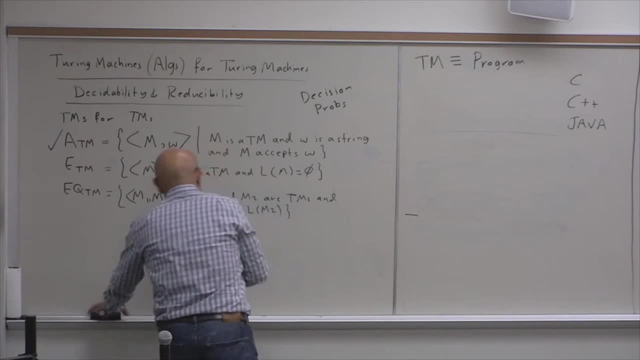 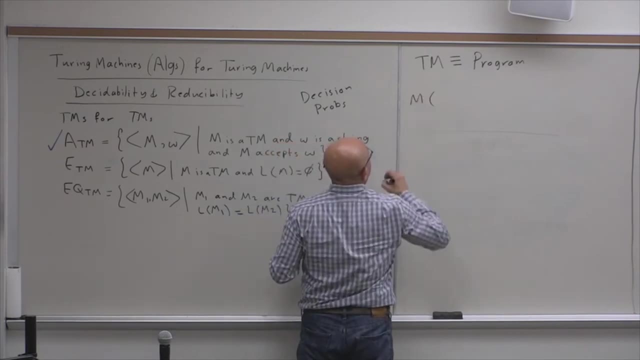 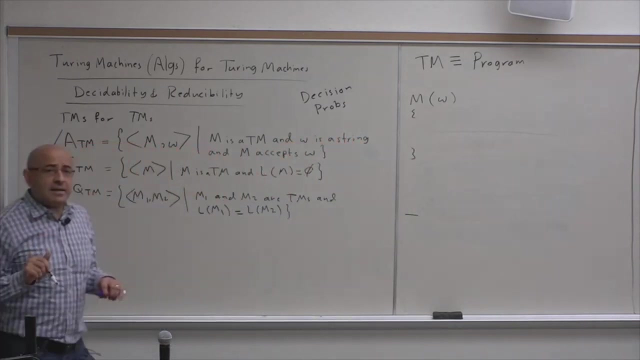 to accept a given string or not. So Okay, So let's look at that. So we are. so there is program M that takes input W And this program M. the idea is that M is a Turing machine or a program written. 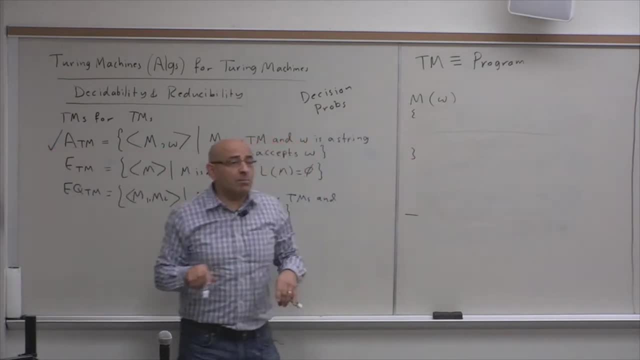 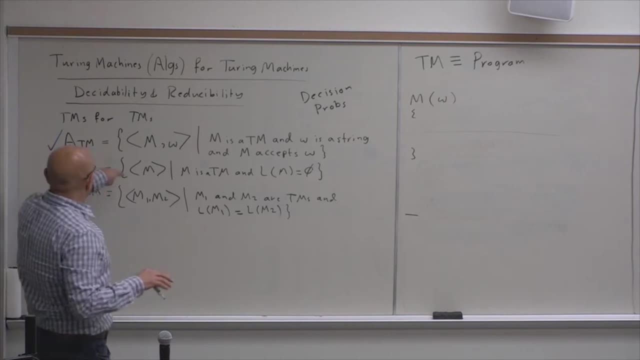 in a general-purpose programming language. So M is a very general program. It can have anything in it. That's why you know analyzing this program is hard. So this is basically. ATM is the program analysis. It's a program analysis tool. 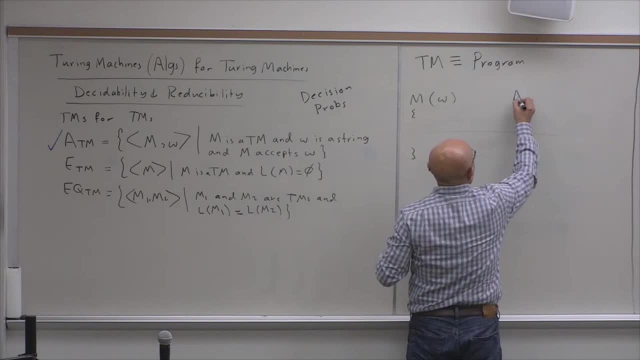 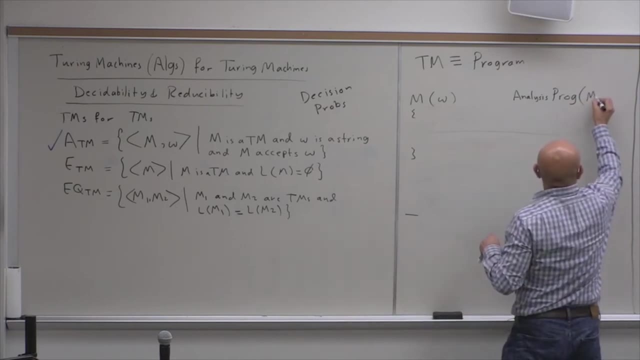 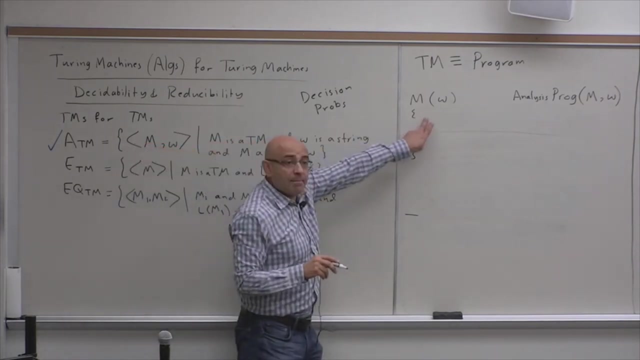 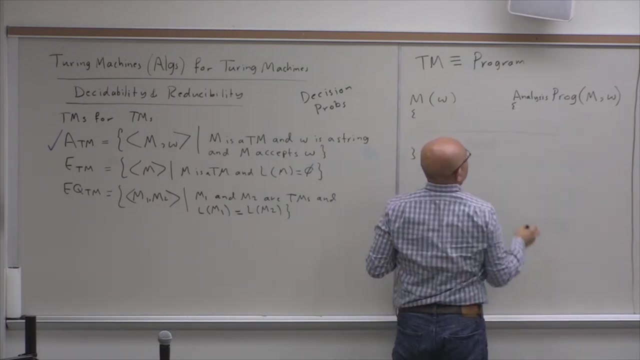 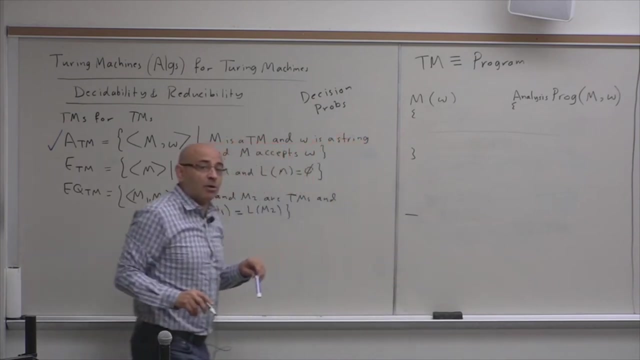 So we'd like to have an analysis tool, analysis program that takes M and W. So it's an analysis program that takes as input another program, M, and the input W to that program, And this analysis program is going to tell us that if we input W into M, the output will be accept or not. 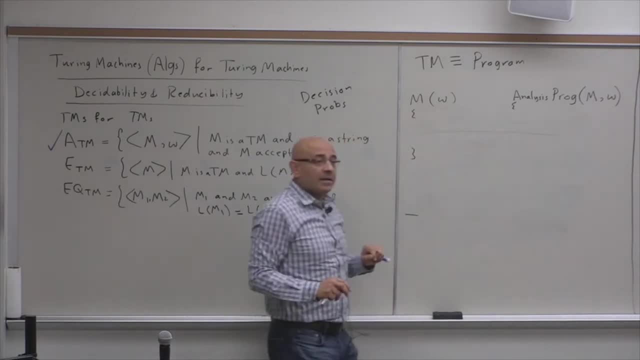 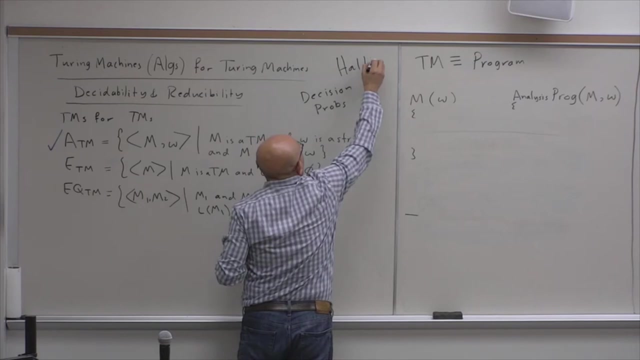 Okay. So now the problem here is that: can this program, can this analysis program, even determine if program M is going to halt or terminate on input W or not? So what if You know, not all programs are guaranteed to terminate within finite time, right? 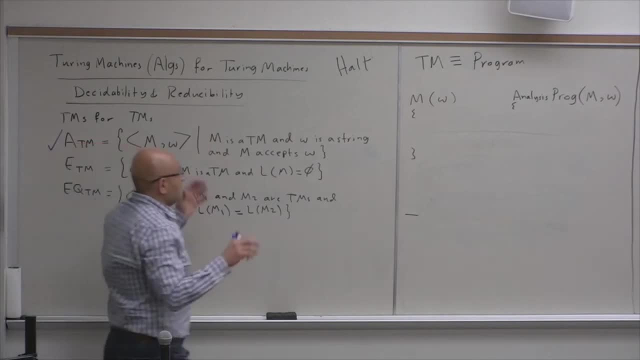 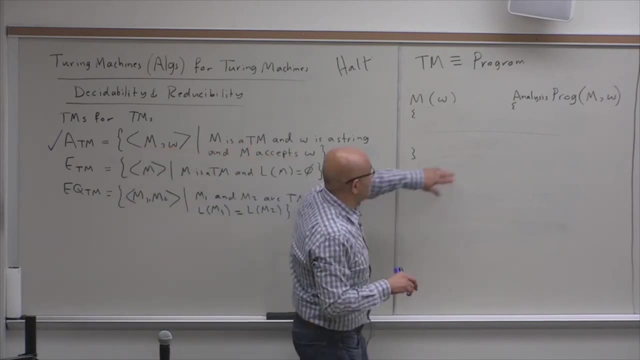 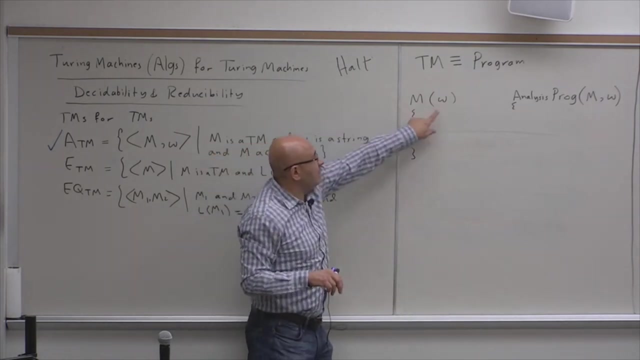 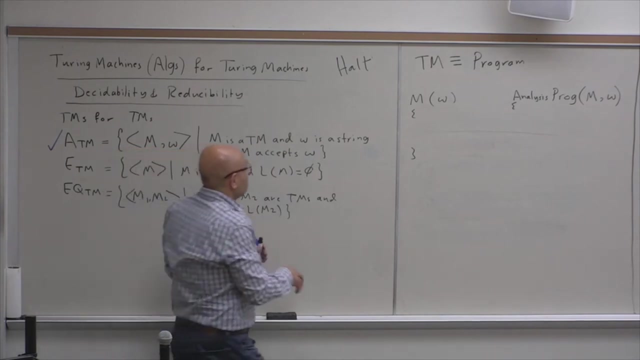 So there are programs that can run into infinite loops. So basically the you know the challenge in writing such a program analysis tool is in determining if program M, when given input W, is going to terminate within infinite time. Now suppose that of course you know for any program M. 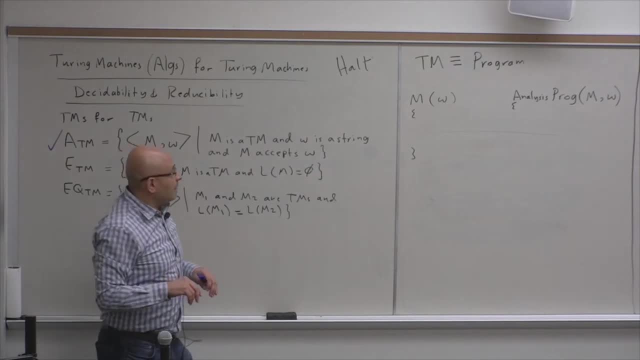 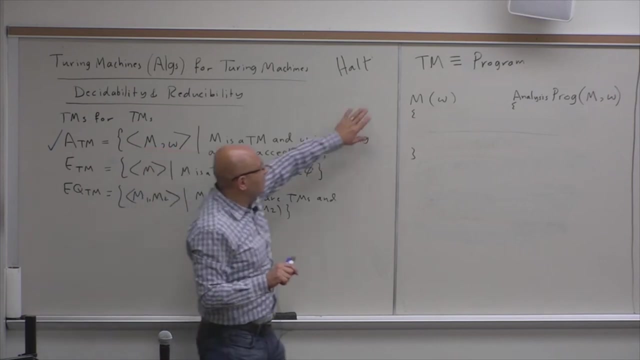 if program M is simple enough, then the program analysis tool is going to know that, you know, is going to know that the program M is going to terminate within finite time. Let's focus on determining if M is going to terminate in finite time or not. 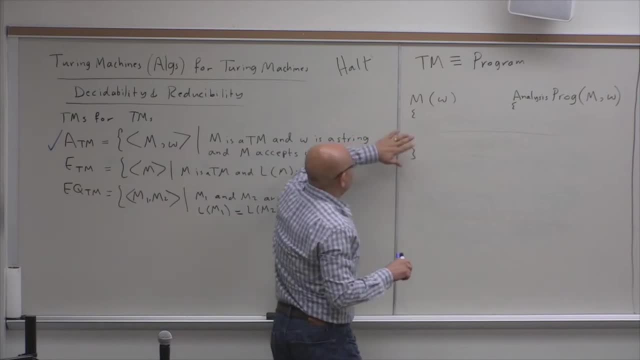 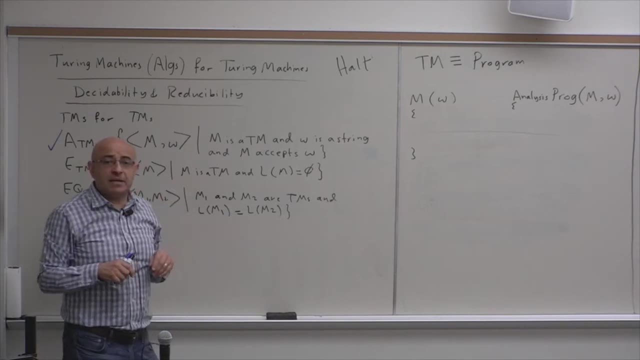 If you know, if M doesn't have any loops, then we know that. you know M has no loops and no recursion, Then we know for sure that program M is going to terminate in finite time. Now, what if M has something like this: 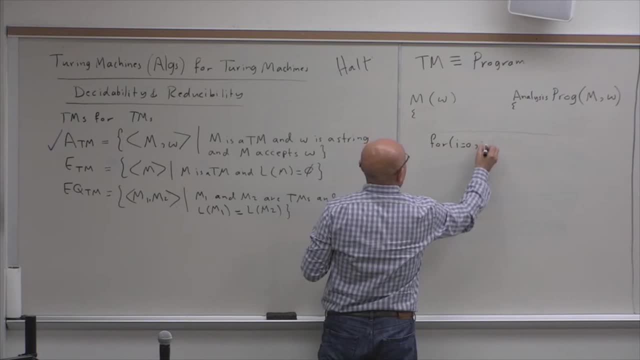 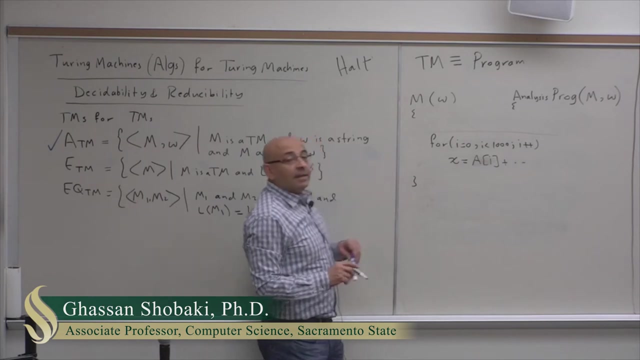 For I equals 0, I less than 1000, I plus plus. and then do something like this: Do something, or you know X equals Y plus, or you know some array reference or whatever. So to analyze a program like this, if you now imagine, 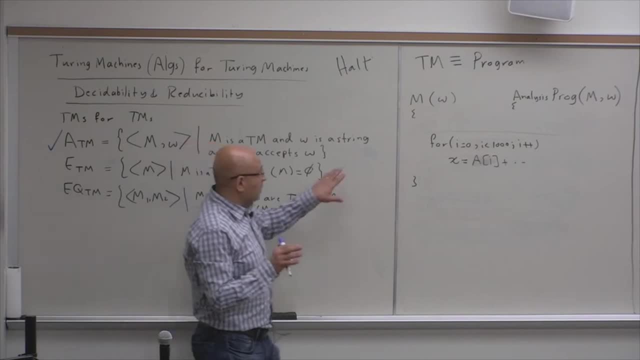 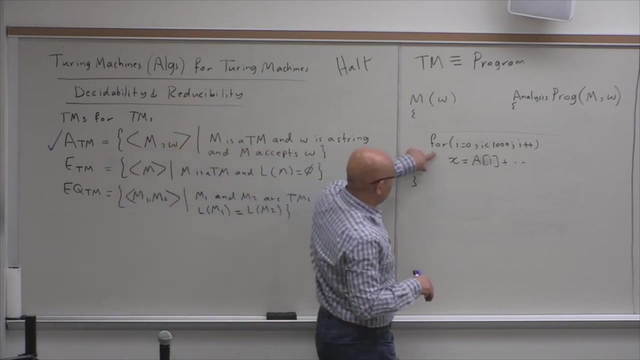 that you are writing an analysis tool that will take this program and determine if this program is going to terminate within finite time or not. Now, if this was the only loop in the program, will you be able to determine? Yeah, So this is, this is the only loop and this only loop. 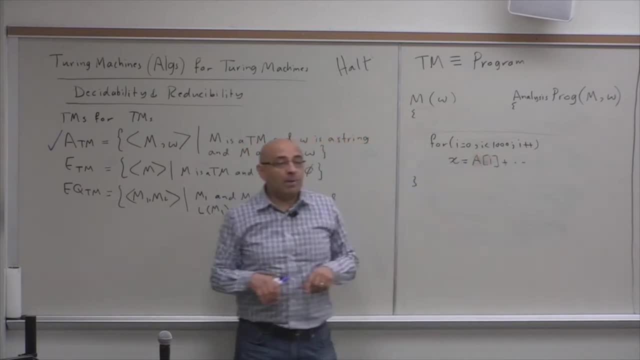 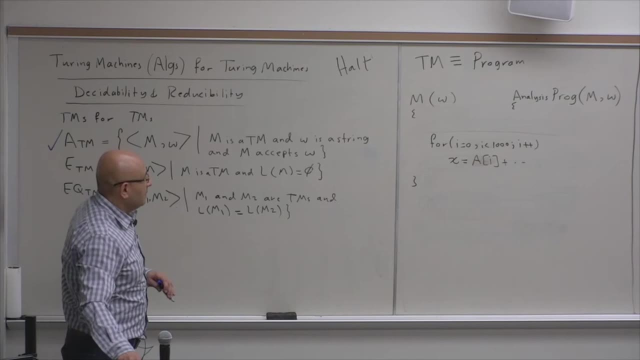 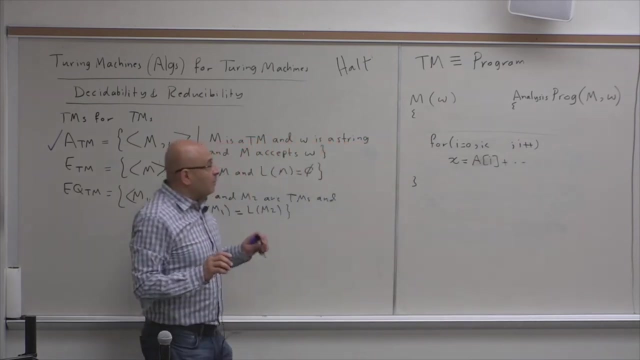 in the program has a finite loop bound right. So it's for an easy program like this. we'll be able to determine if it that it will determine within finite time. Now, what if we have this? Now, the thing is that we are we're looking for an analysis tool. 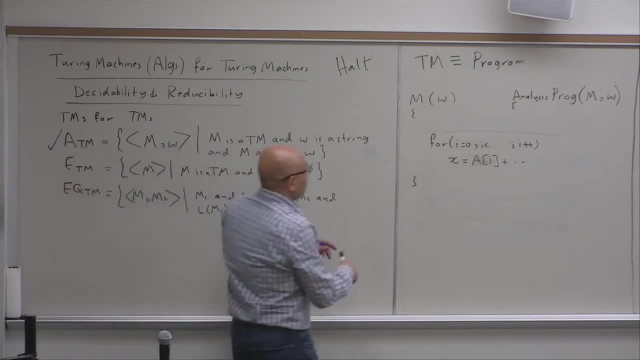 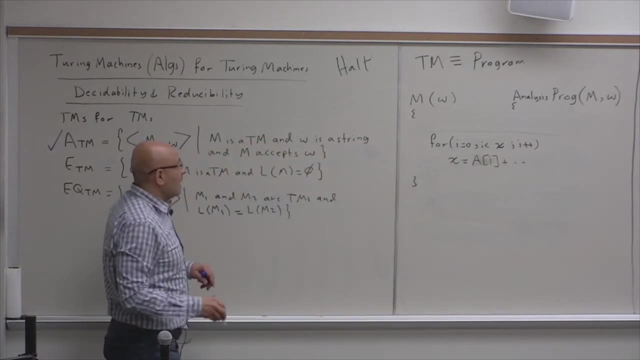 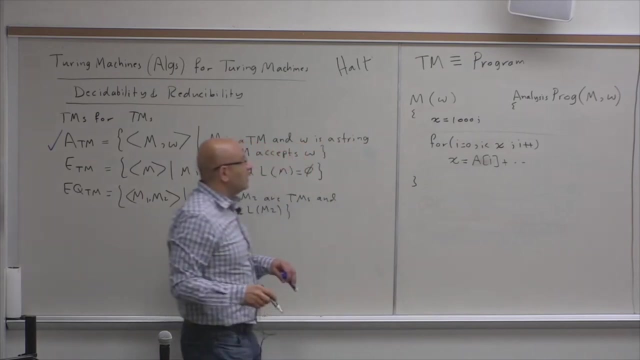 that can analyze a general program, right? So a general program may have something like this: Now, if X equals, if you have somewhere X equals something- 100 or 1000 or whatever- then again, this is something that you can analyze. 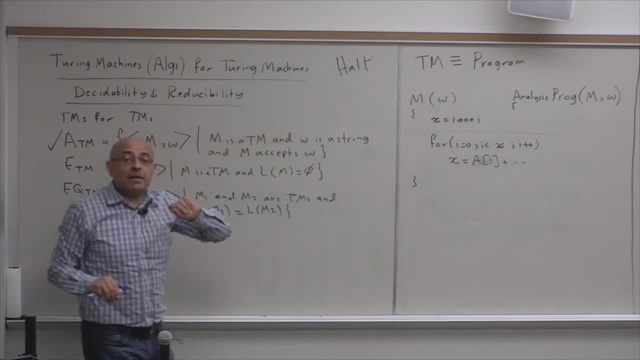 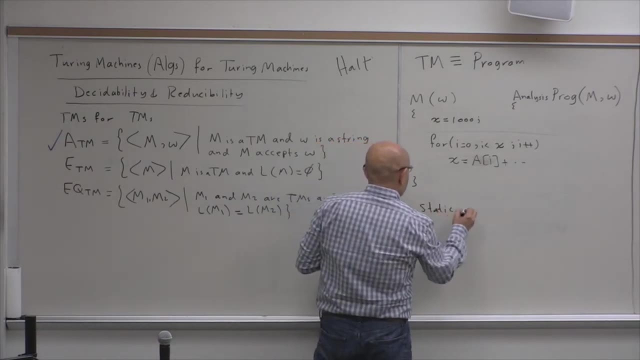 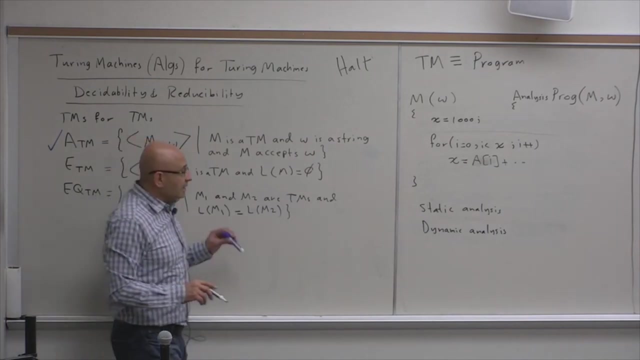 Now we're trying to analyze the program at compile time, without running it, without running the program. So we have the notion of a static analysis of a program And a dynamic analysis. Now, what's a static analysis, Analysis at compile time Or analysis without running the program? 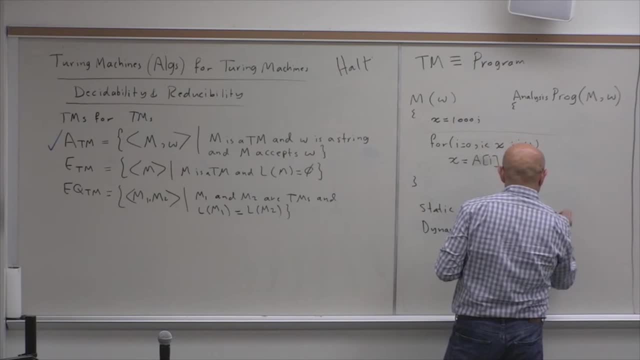 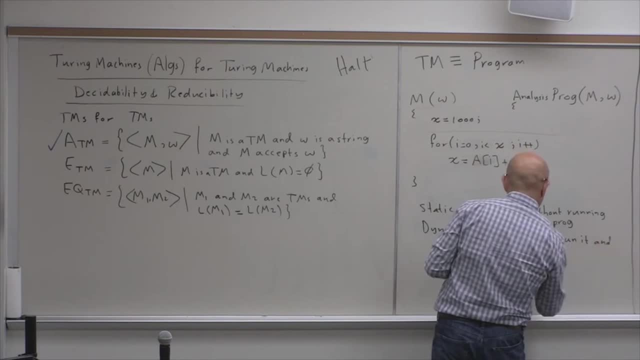 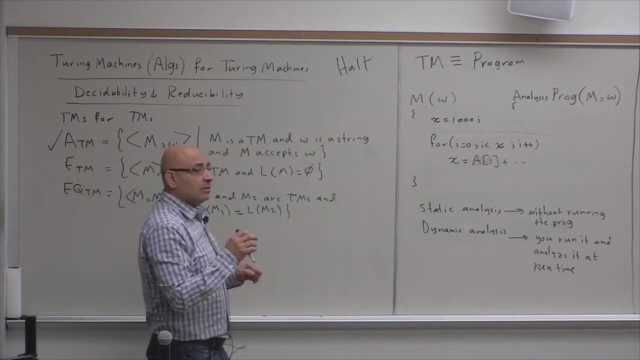 and analyze it at runtime. Now, how many people have used program analysis tools? Okay, So what program analysis tool? Claim time? What's that Claim time for a? Okay Checking for What does it check for? Codes known as equals to. 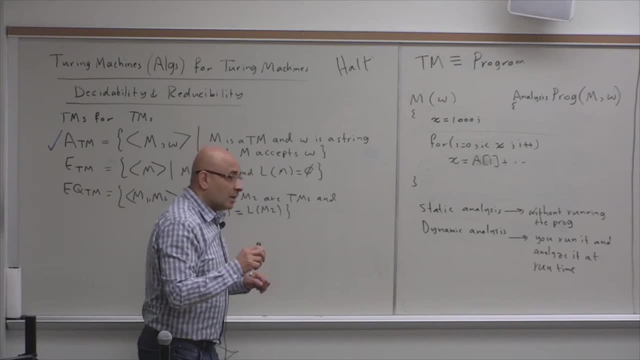 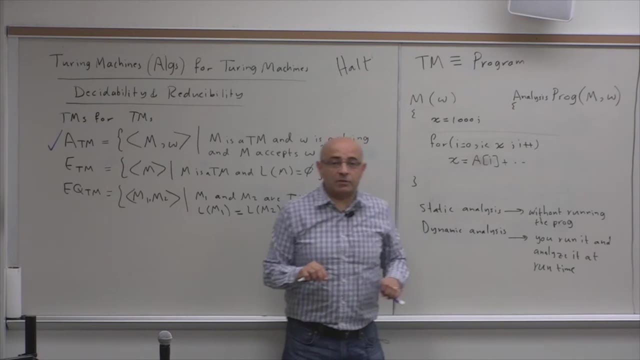 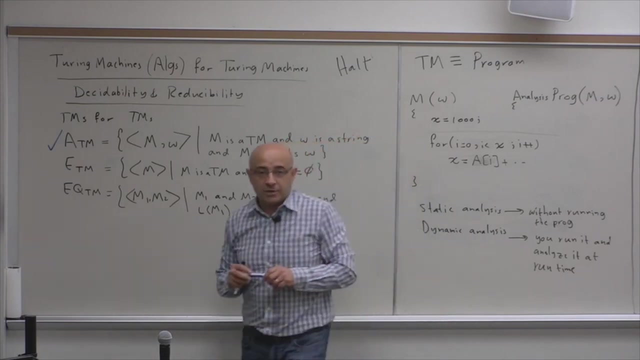 Okay, Okay, Is it static or dynamic? Yeah, So it's static. It means that it takes your code and analyzes your code and gives you some information, like you know, checking for uninitialized variables, for example, Okay. Or checking for out-of-bound memory accesses. 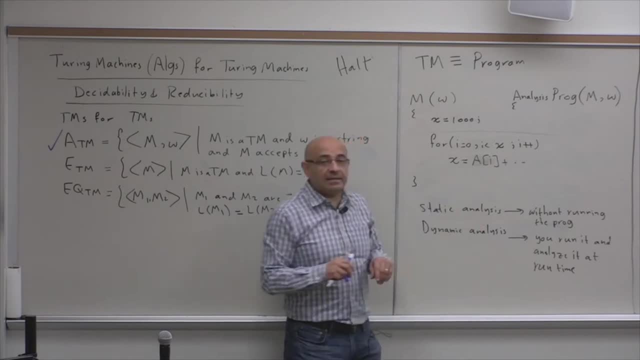 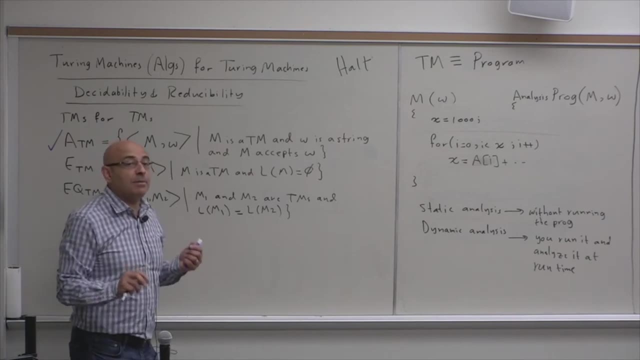 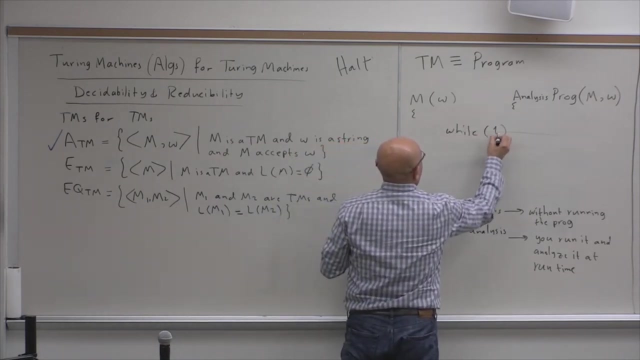 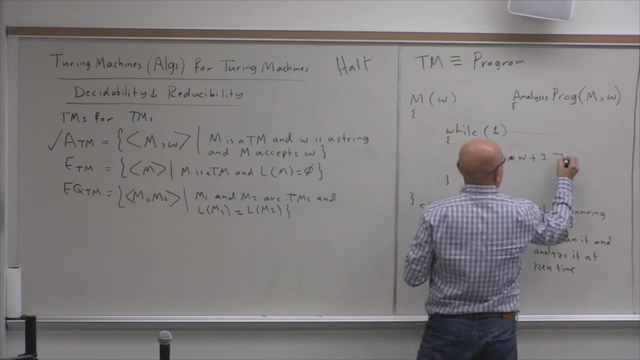 Now, some of this can be done with a static analysis, but not everything can be done with a static analysis. Why? Because it's the behavior of the program: is input dependent. Now what if you have something like this And then if 2 times W plus 3 is greater than 5 brink? 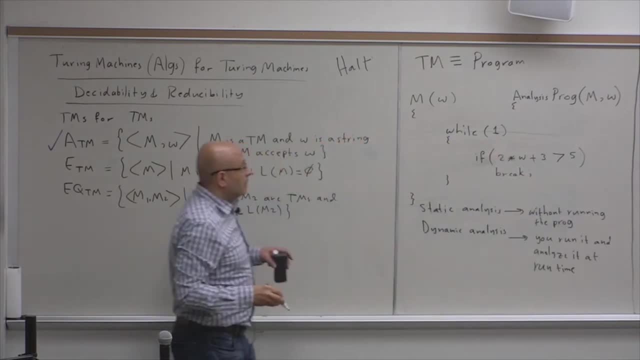 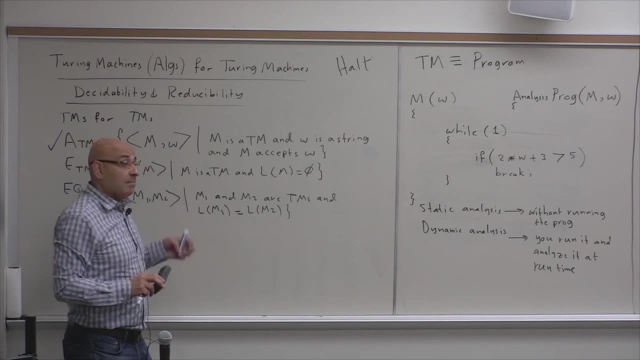 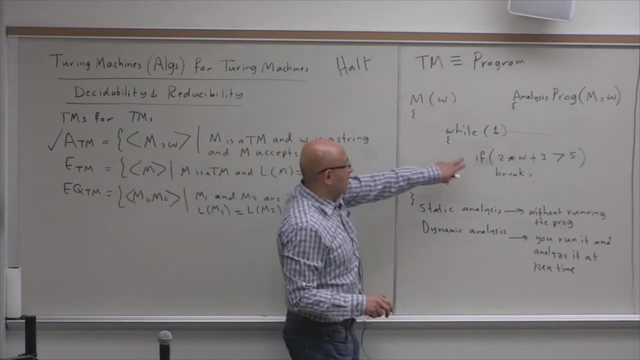 Now, can you determine with a static analysis- you know without running this program, whether this will terminate in finite time or not. In fact, can you determine if this condition will ever become true? Why not? Because it depends on W, It depends on the input. 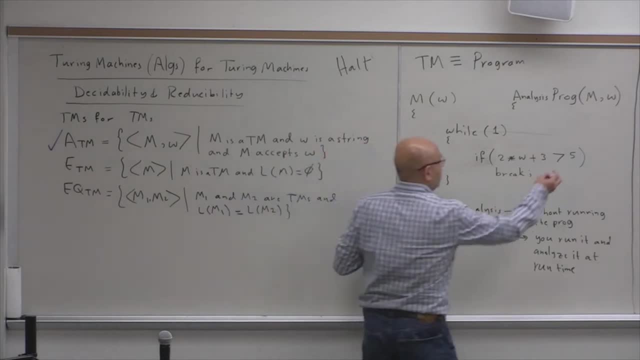 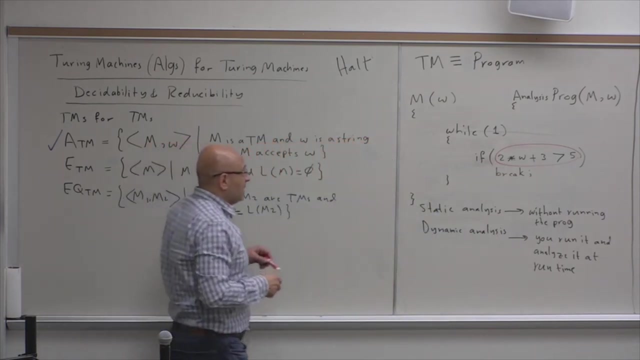 and we don't know what that W is. Okay, So here this is an expression that uses W, and this expression determines if the program will terminate in finite time or not. But things cannot be, you know, may not be as simple as that. 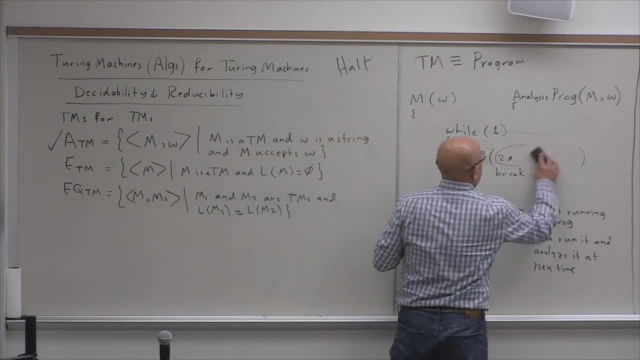 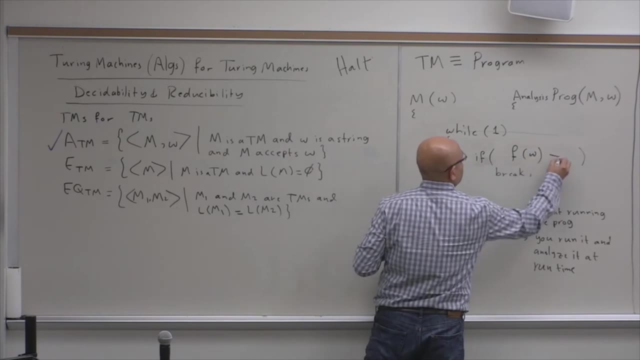 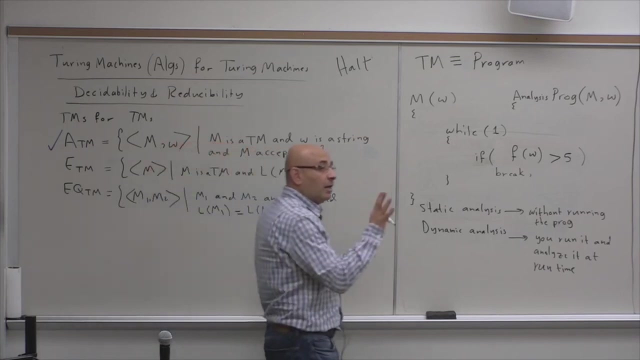 You can have something like you know F of X function- It's called the function F that takes W, And then this function can be anything. You know this is a general purpose programming language. We're trying to develop a tool that can analyze any program. 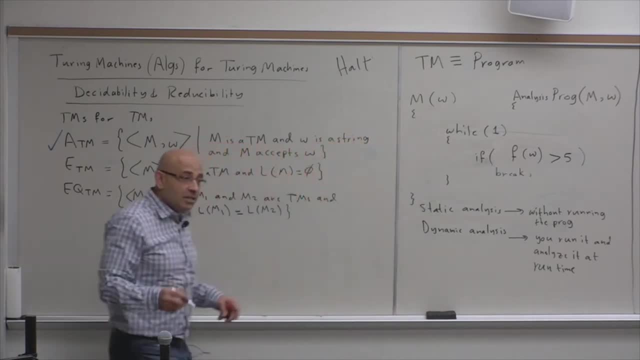 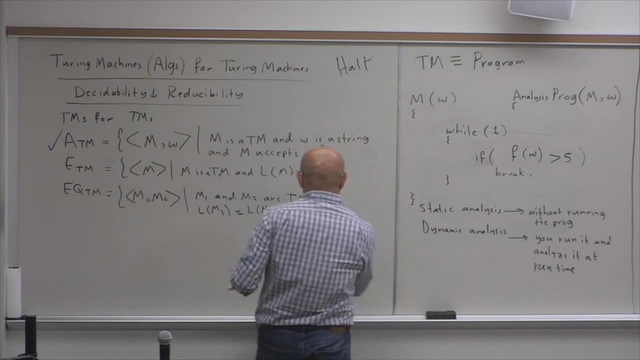 And then in this F, this F can call G, and G can call H, and H can call whatever. So there can be a whole sequence of function calls. So function F is going to call function G, and then function G can call function H, And you can have a. 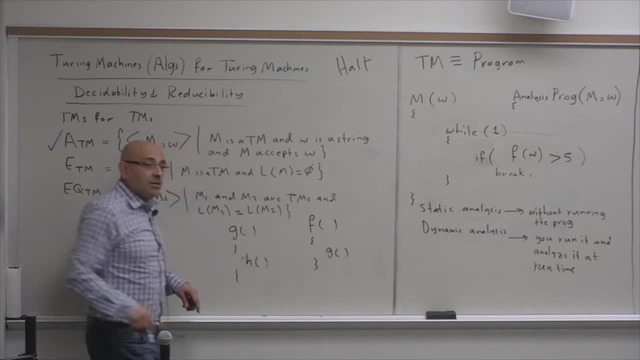 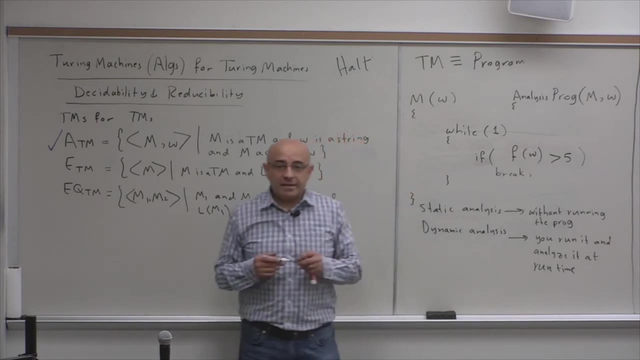 whole sequence of functions called. So function F is going to call function G, and then function G can call function H And you can have a whole, you know- sequence of function calls. So this is the bottom line. is that with a static analysis, 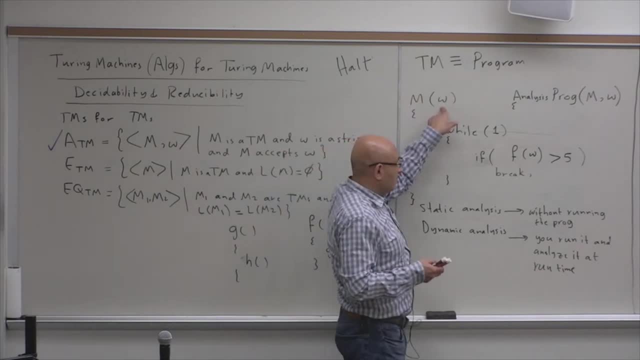 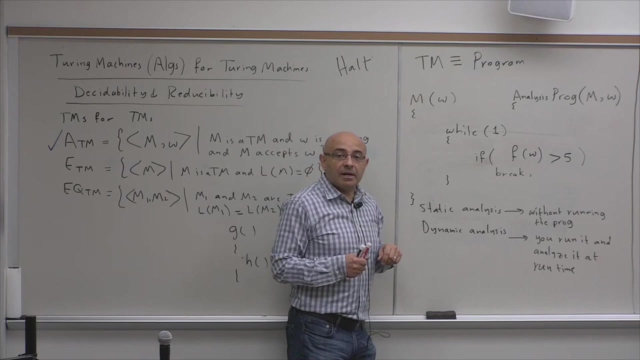 without running the program on input W, you will not be able to determine if this program terminates in finite time or not. If this program is guaranteed to terminate in finite time when you input W or not, Right? So then, in fact, this is the ATM program. 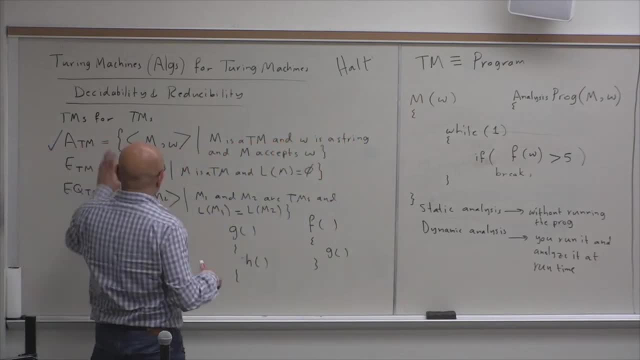 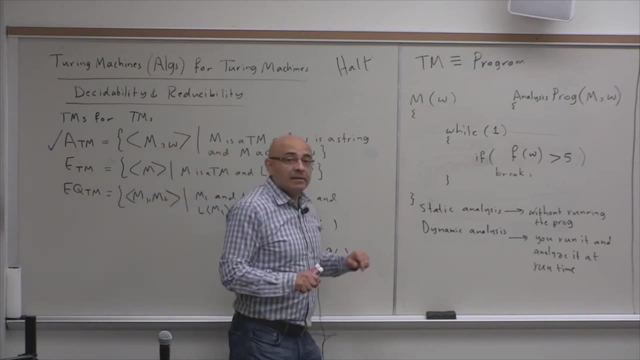 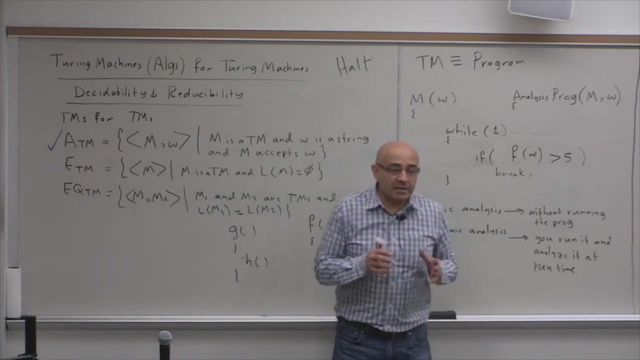 Right. Yes, This is the ATM problem. It's in order to determine if a Turing machine accepts a string or not. you will need you know. an important part of this is determining if that Turing machine is going to halt, is going to terminate within finite time or not. 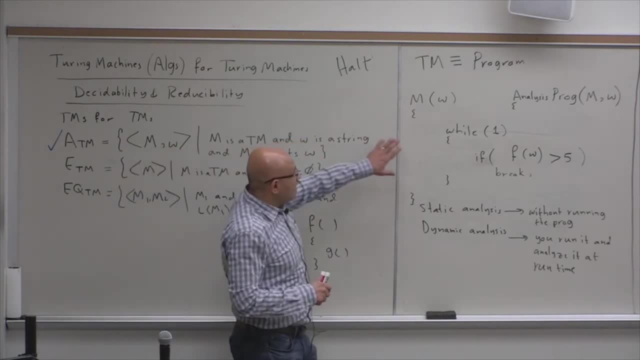 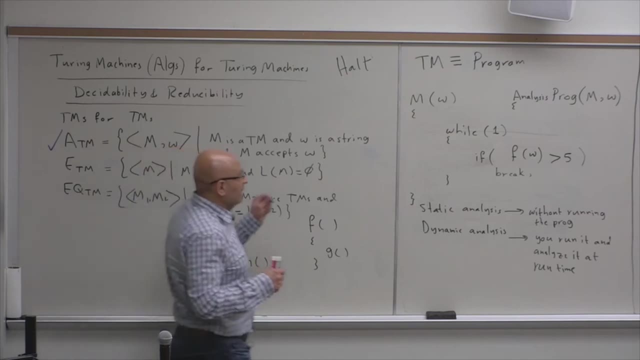 And with a static analysis. you know, I hope that I convinced you intuitively that with a static analysis you cannot determine if a program can terminate within finite time. You will need to do a dynamic analysis, And a dynamic analysis in this case would be just. you know. 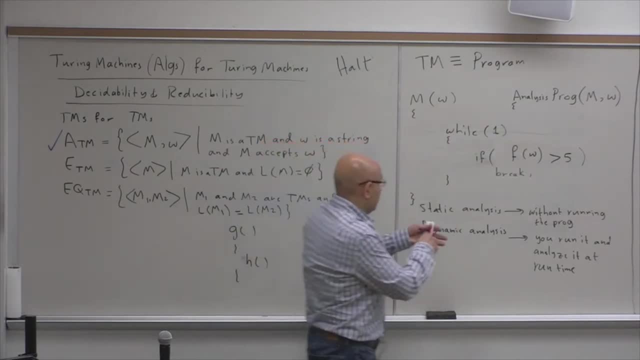 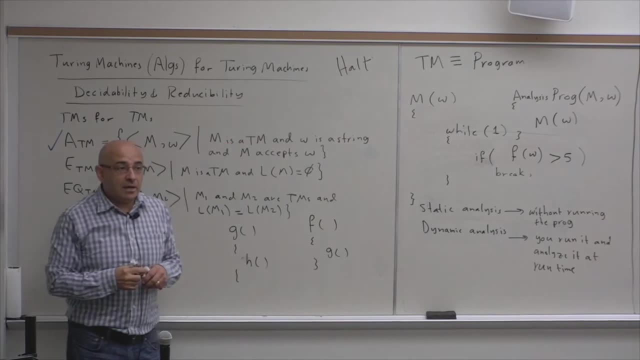 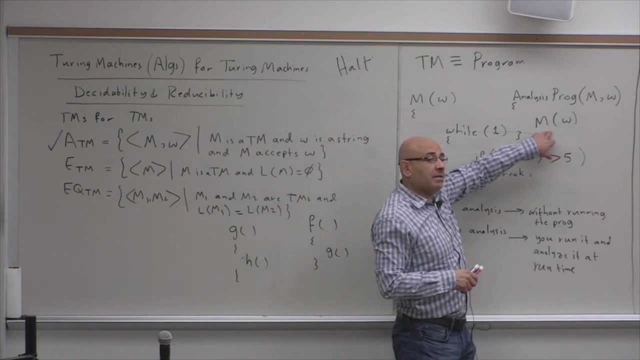 this program analysis tool is just going to run M, Just it's going to invoke M on W, So you know a program can run another program, Right? So in how many people have written programs that run other programs? 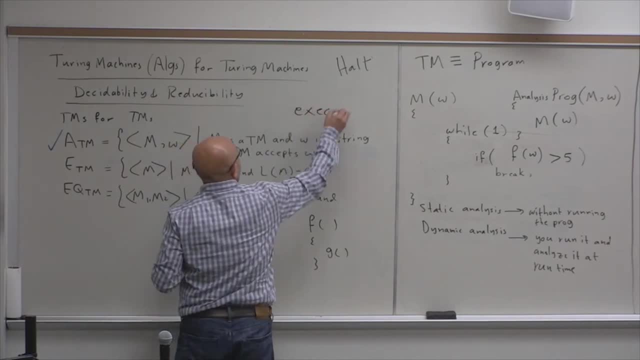 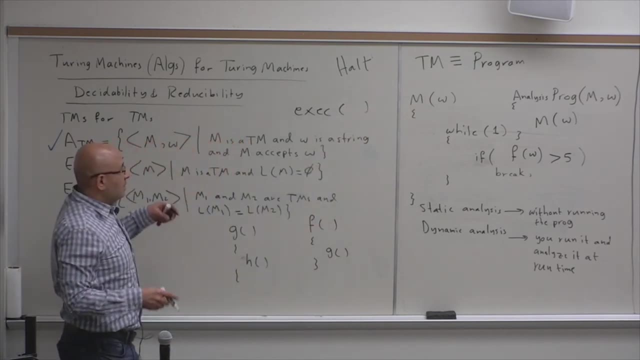 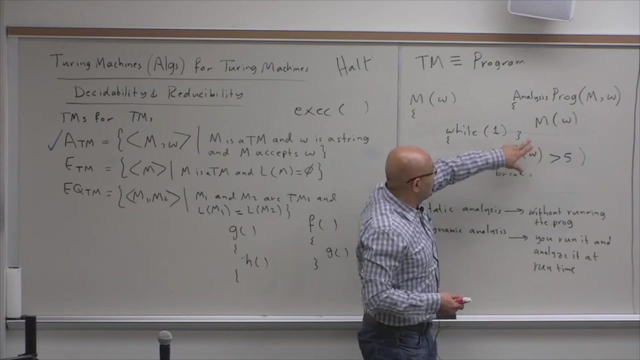 Yeah, So you can. you know you, on Linux you have the exec function call that can execute another program, And so there is a system call that will allow a program to run another program. So if this program analysis tool is going to run this program M. 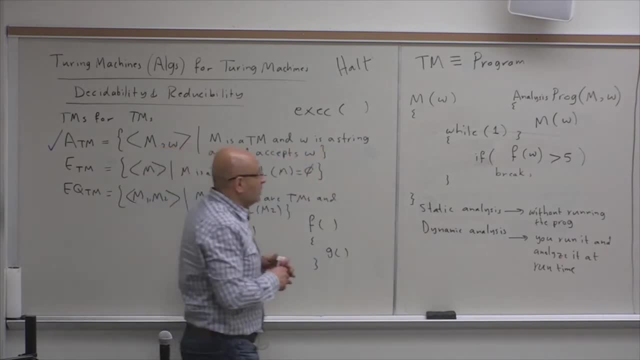 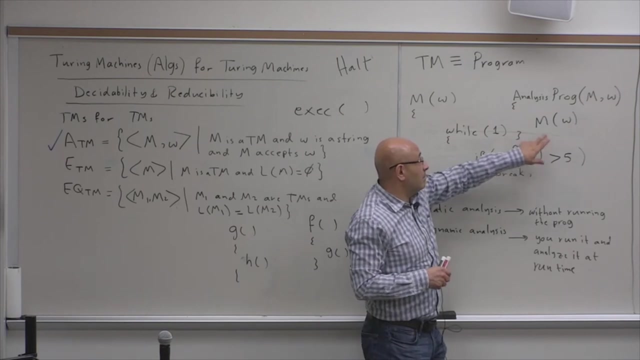 and then to determine if M is going to terminate within finite time or not. Now, is this a decider? Is this a? is this a Turing machine that decides the problem? No, it doesn't decide the problem, because if M runs, 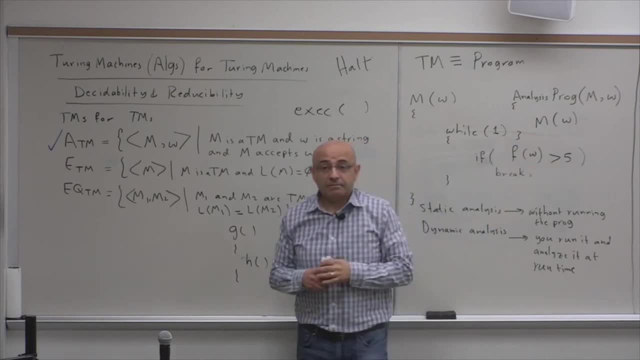 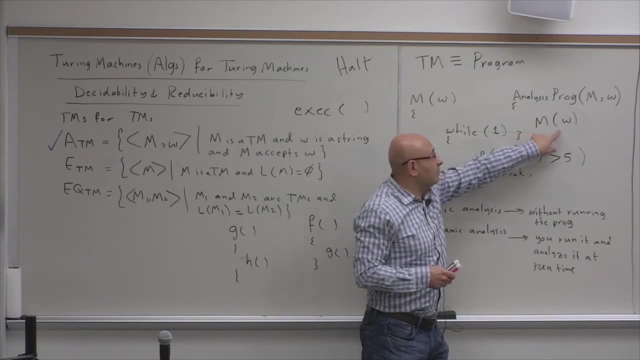 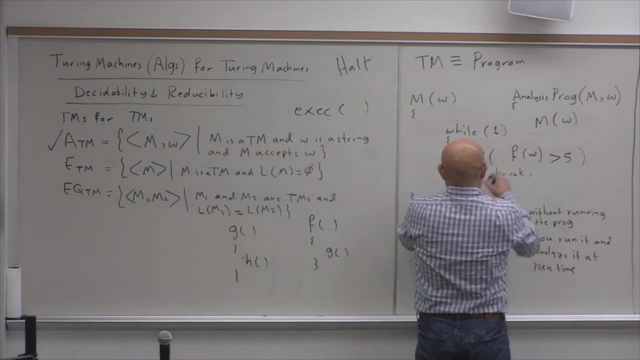 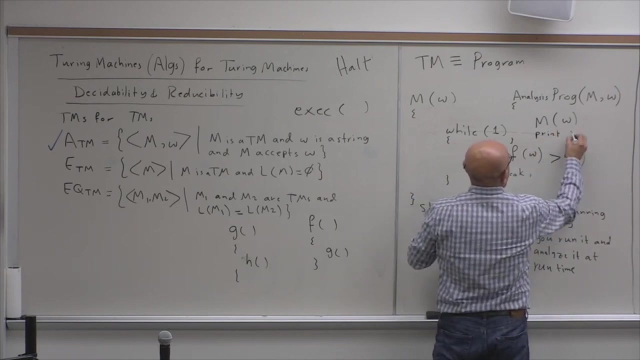 into an infinite loop. M will never return. Right Now we know that if M doesn't run into an infinite loop with input W, we know that M is going to return. and then here we know that M is going to print. you know, print yes. 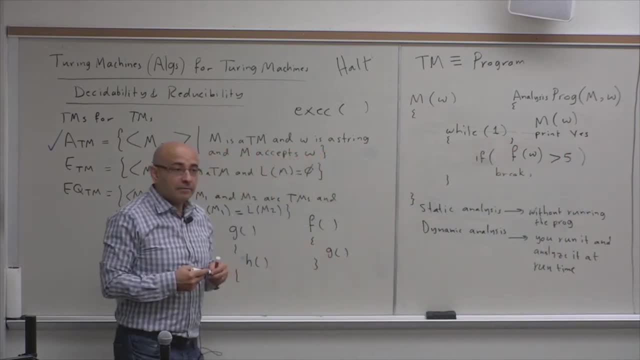 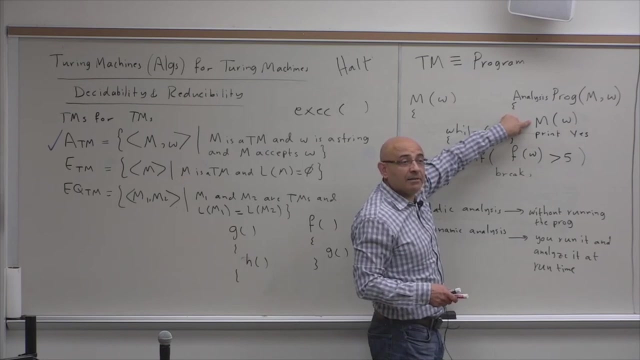 So we're trying. you know, this analysis program is trying to determine if M terminates in finite time or not. Now it's going to print yes if M terminates, but if M does not terminate, this yes will never be reached. 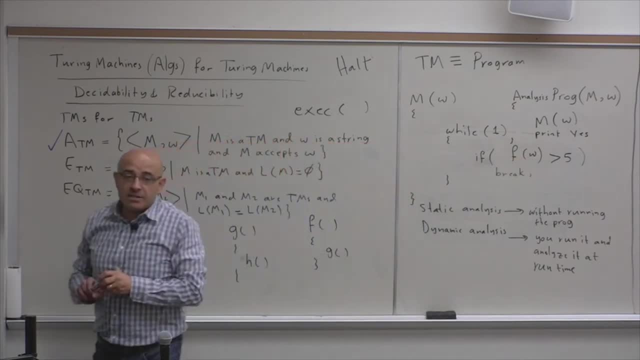 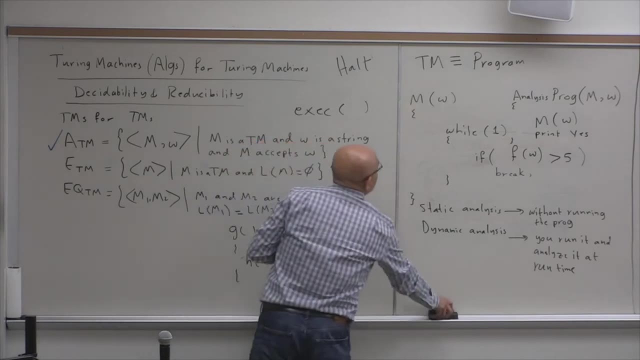 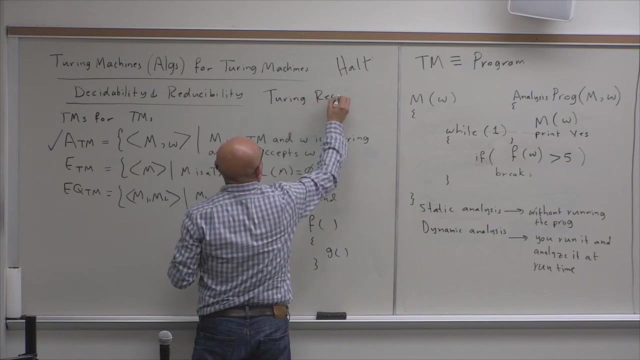 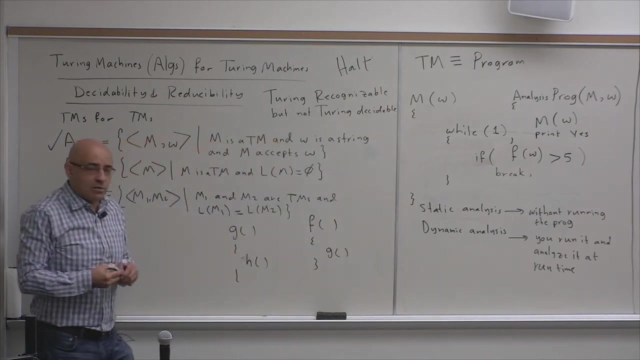 Right. So this is exactly what it means for a problem to be Turing recognizable but not Turing decidable. So this problem is Turing recognizable but not Turing decidable. You know, again, a Turing machine is a problem. So, in other words, you can write a program. 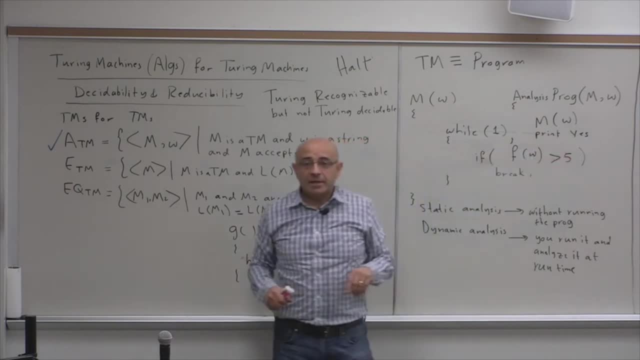 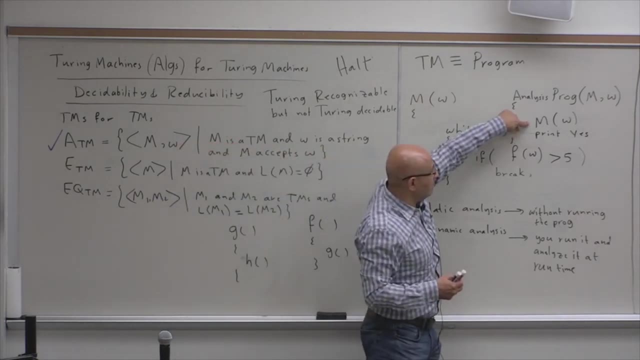 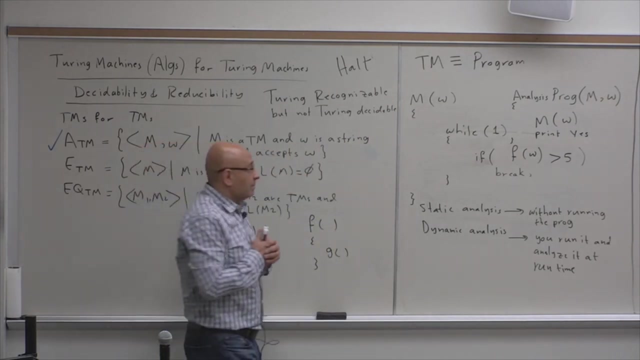 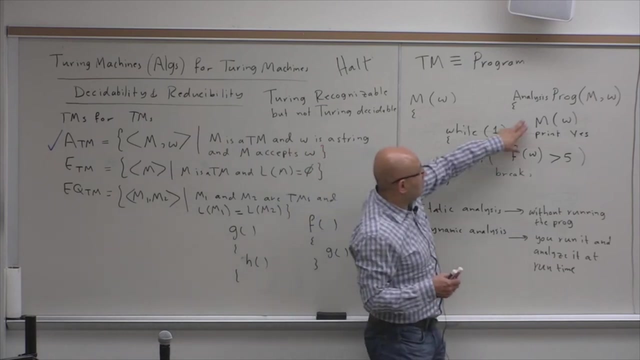 you can write an analysis program that takes another program and determines if it terminates in finite time or not. If that program terminates in finite time, on that input the program will print: yes, and it will terminate in finite time. But if this program runs into an infinite loop, then what? 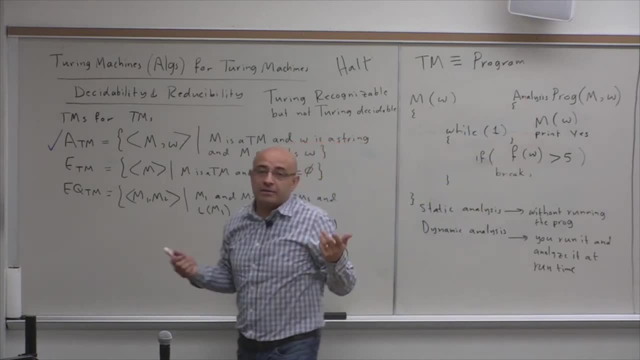 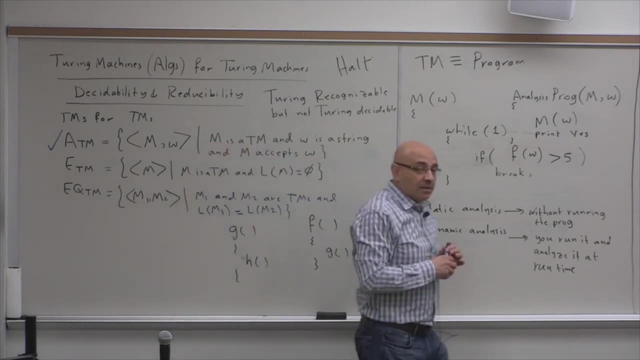 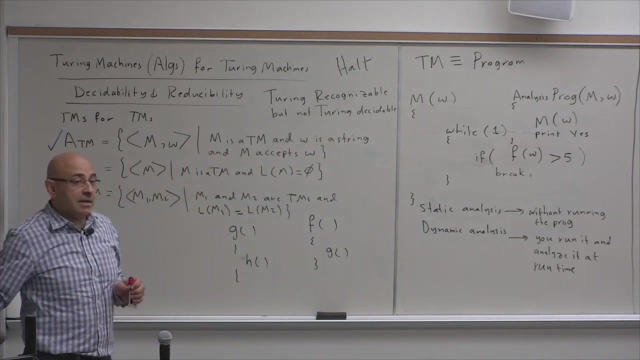 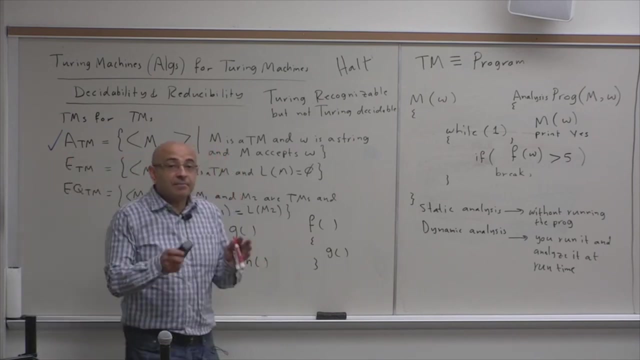 Then the analysis program itself will not terminate. So that's why this is the intuitive explanation that this problem is not Turing decidable. You cannot come up with a Turing machine or an algorithm or a program that does this. that can take an arbitrary program. 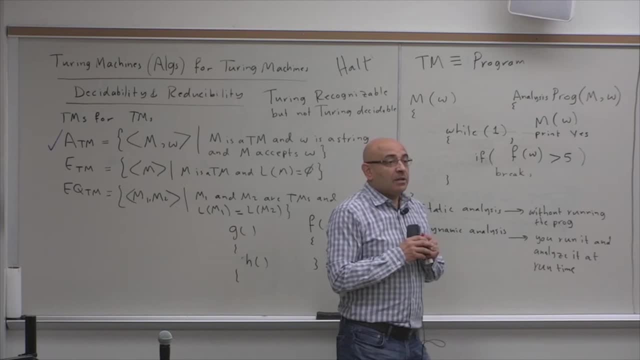 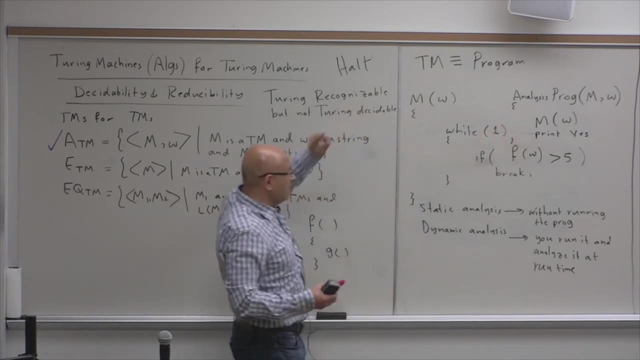 that's written using the same general purpose language. So here the idea is that this program M is written in the same general purpose language, And because it's written in the same general purpose language it can have anything. So it can have this function F, Its termination is dependent. 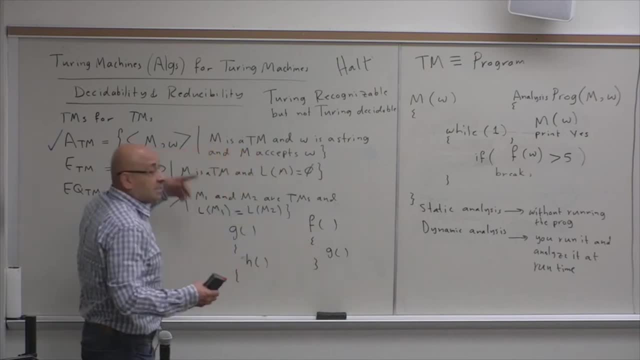 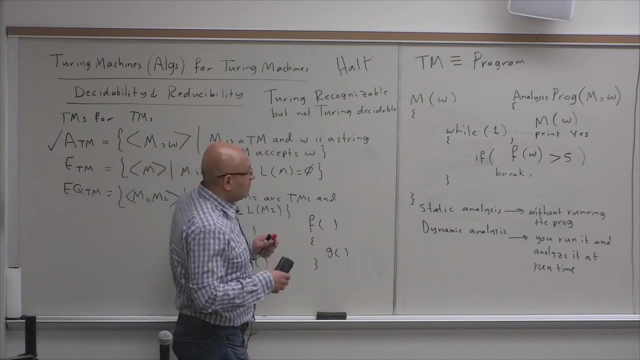 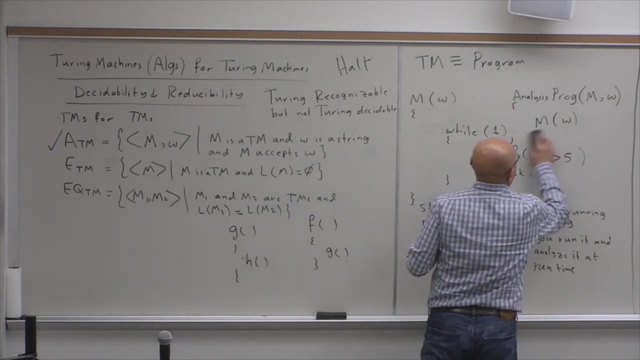 on F, And F is dependent on G, and G is dependent on H, And this dependence chain is not bounded by anything. Okay, Now, this is determining if it holds or not. But here, you know, this is the you look at the return value. 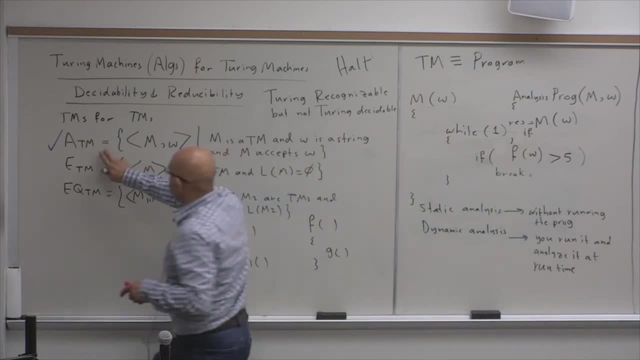 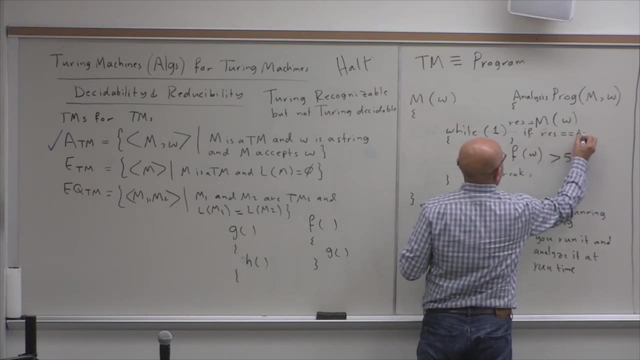 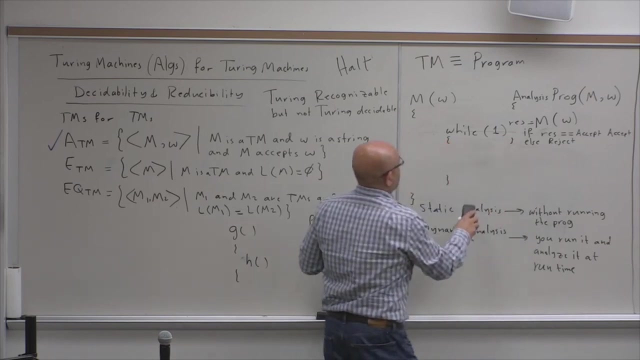 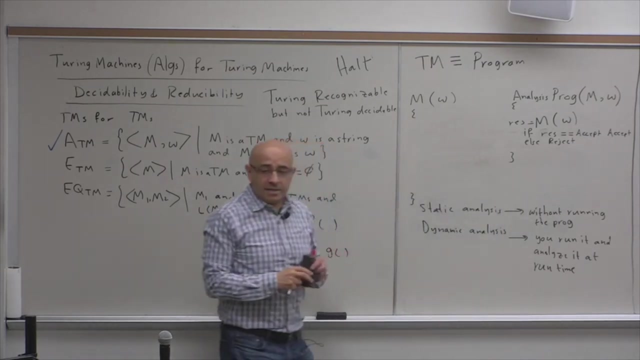 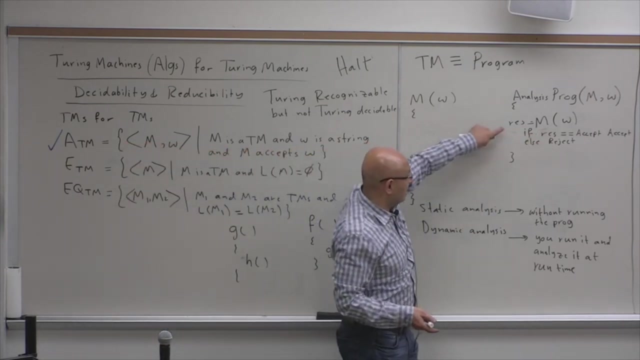 the result. so solving this problem, the acceptance problem, if M or if result equals accept, accept, else reject. So this, this program, this analysis program on the board, this is a dynamic analysis tool that takes any program, It simply, it simply runs that program and looks at the result. 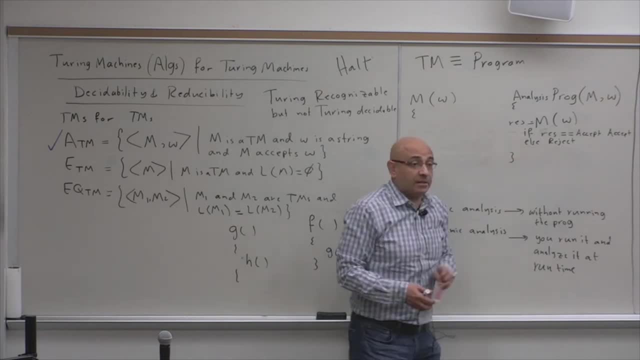 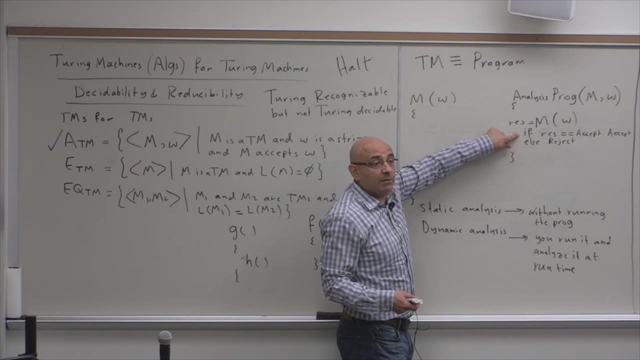 If the result is accept, it accepts. If the result is reject, it rejects. But the problem with this is that we are not guaranteed that this if statement here will ever be reached, Because if this guy runs into an infinity, this infinite loop F will never be reached. 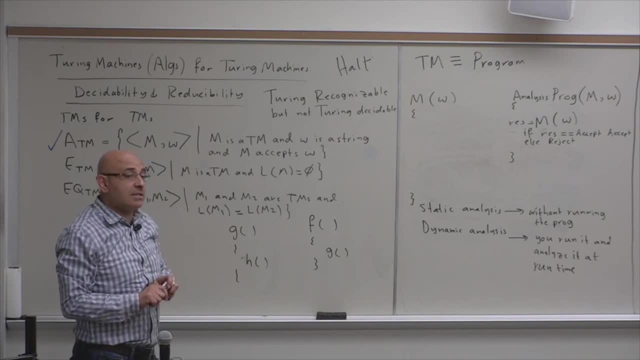 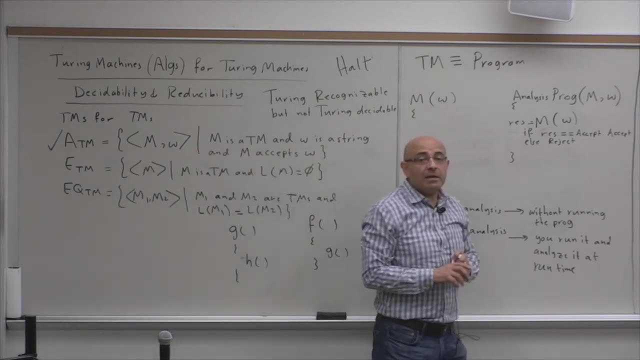 Yeah, so that's the dynamic analysis. The dynamic analysis is just run the program that you are trying to analyze. So you run it. but again, the key issue is that it's not guaranteed to terminate. It may run into an infinite loop. 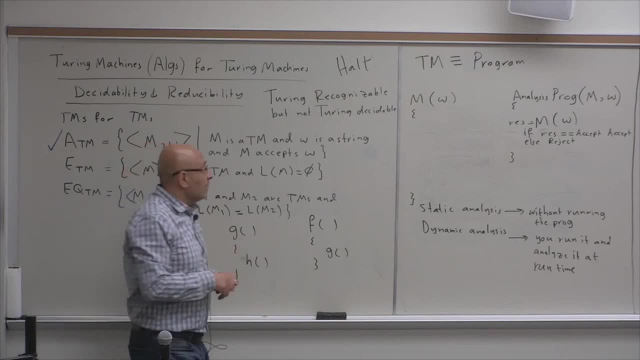 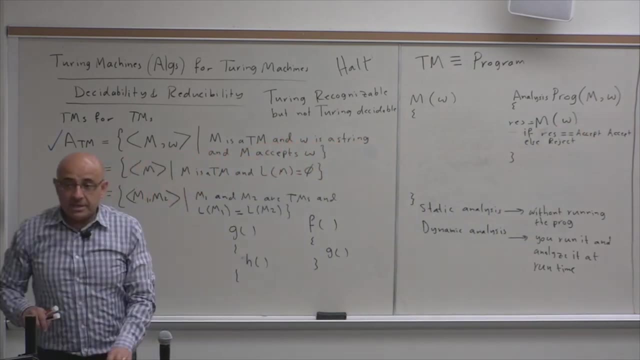 And if it runs into an infinite loop, you will never know if it accepts or rejects string double. So this is an intuitive explanation. So there is a. there is an actual proof in the book. So we'll not, we're not going to do the proof. 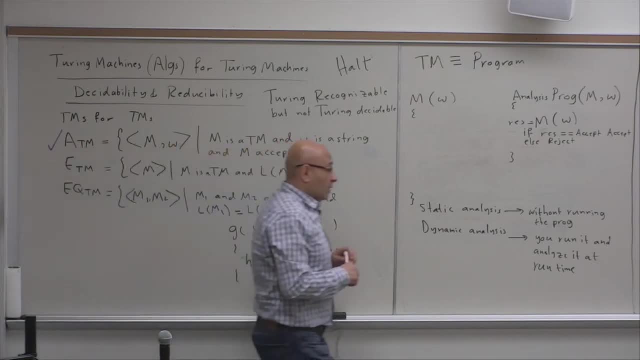 the abstract proof for this. You know you are welcome to look at this, But you know of course you are in the tests and in the homework. you're responsible only for what we explain in class. So in class we're not going to do the. 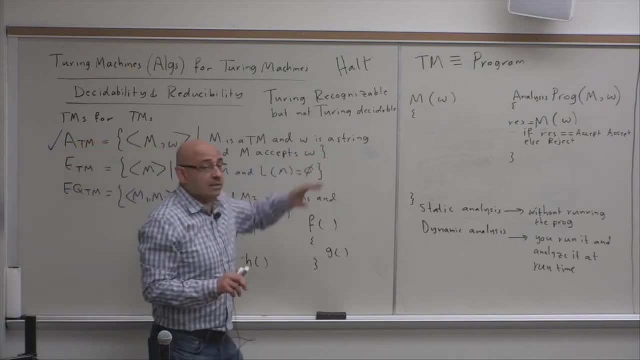 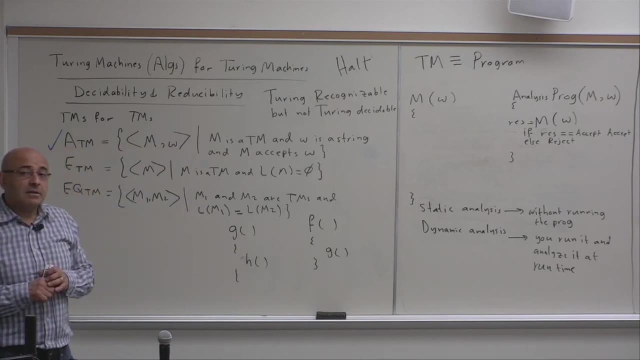 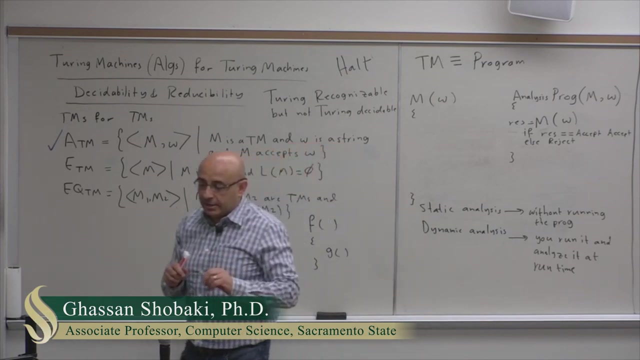 the abstract proof. You're only responsible for understanding this intuitive explanation. Any questions on this? Okay, So the bottom line is, if someone asks you to run a tool and to write an analysis tool that will take an arbitrary program and determines if that program has an infinite loop in it or not. 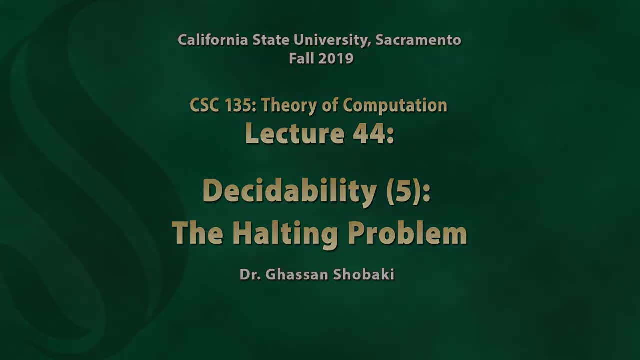 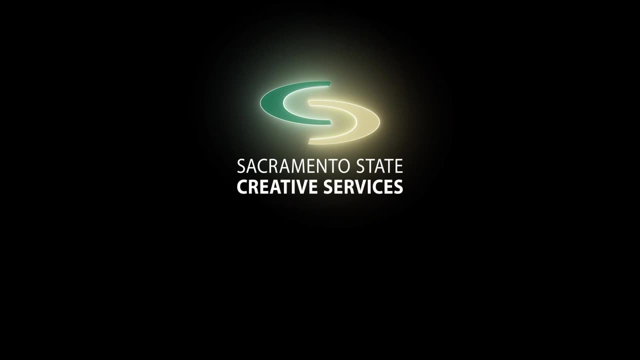 you will not be able to write such a tool. So you will not be able to write such a tool. So you will not be able to write such a tool.